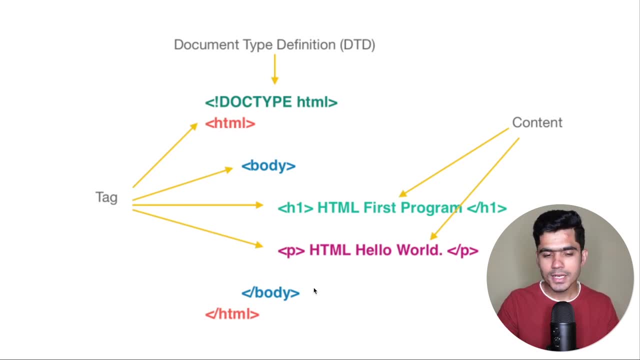 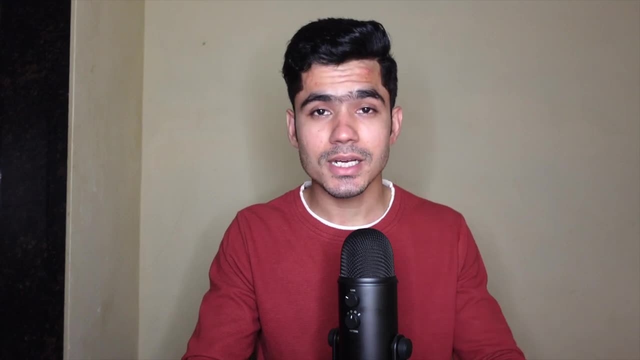 then you write everything inside the body tag. There are different tags available, such as H1 tag to display header, P tag to display paragraphs, And there are so many different tags available If you want to increase the size of the font, if you want to make it colorful, and so many different. 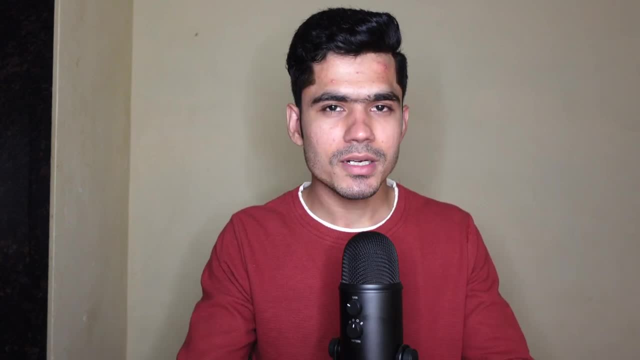 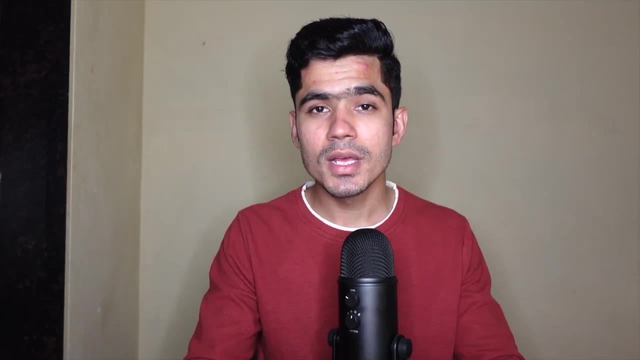 things, So we are not going to deep dive into HTML. If you want to understand the basics of HTML, I will suggest you to go to the WC school. I will give you some of the basic strategy that you can use to understand the HTML code and scrape data from the website. 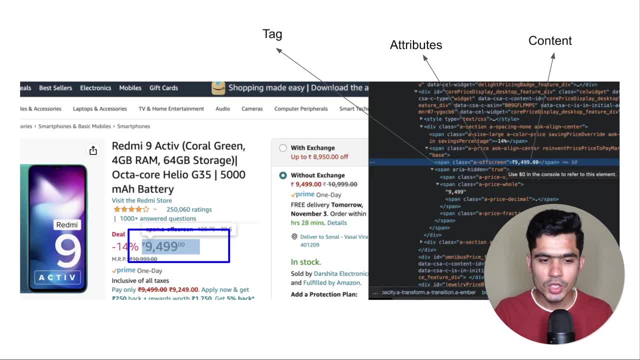 So let's start by understanding the basic structure of Amazon website. So if you want to understand this price and how it is displayed on the Amazon website, you can directly go and check the code and I will show you how to check the right code for right. 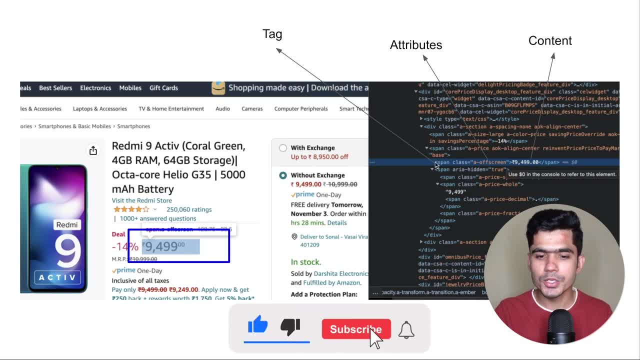 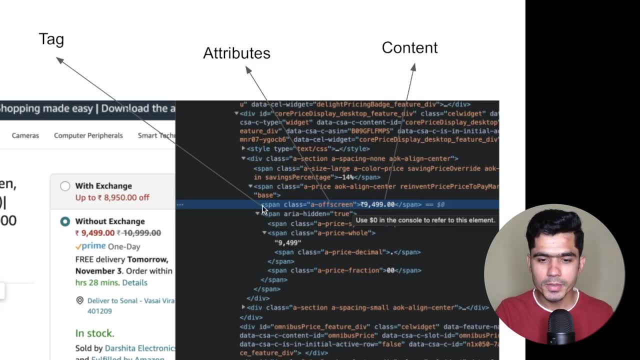 particular element, But for now just understand that this is the code that is being used to display this price number. So over here we see three things. One is a span. Okay, Span is a tag available in HTML. Second thing we have over here is attribute. And third thing is the content. 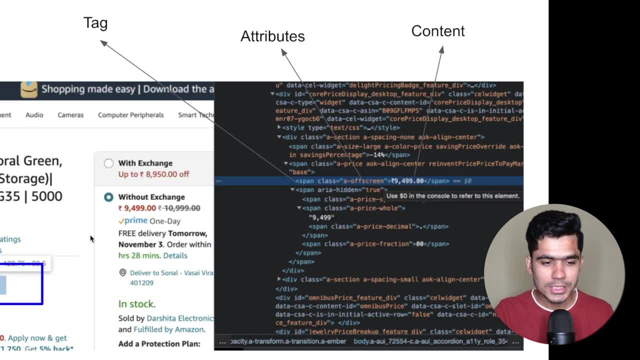 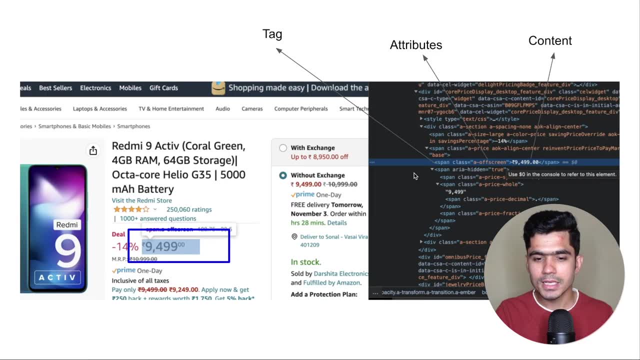 the text that you want to display on Amazon website. So, as you can see over here, the 9,499 is displayed over here, but the text size is big, So that kind of formatting is happening inside the attributes. So there will be a one class store inside the CSS. 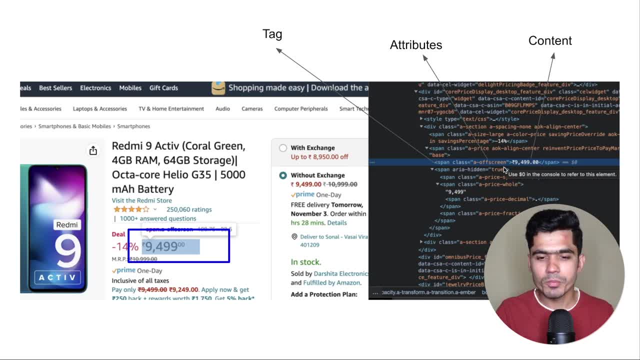 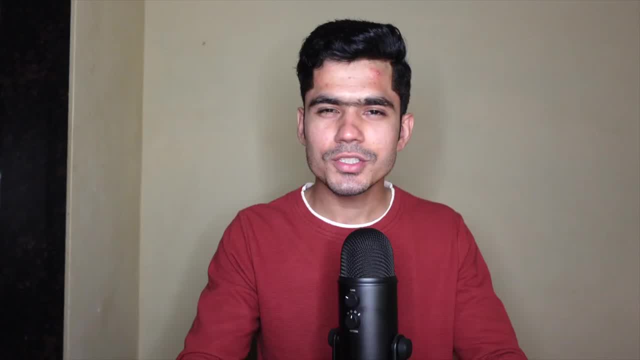 a dash off screen, That is, that contains all of this information. Now, to scrape data, you don't have to understand this code. You just need to get the right information and put that in your Python code. So let's talk about the basic prerequisite required. 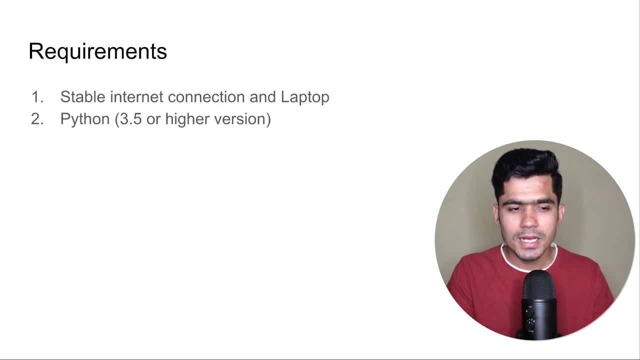 for this project. So number one thing you need is stable internet connection and laptop, And second thing, you need to install Python 3.5 or anything higher than works fine. So if you don't have Python, I have the tutorial already. I will put the link in the description. 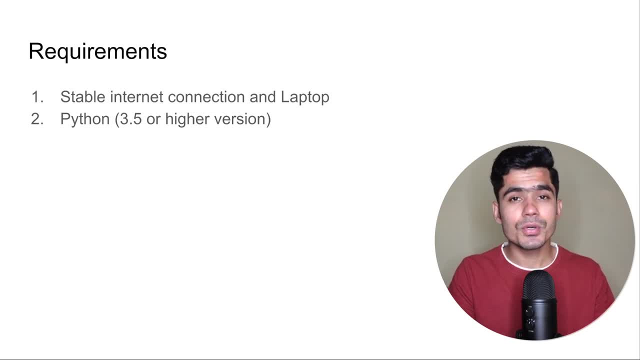 You can go and watch the tutorial and install it. Second thing you need to do is install the Jupyter notebook. In that tutorial I've explained how to install the Jupyter notebook also, So go there, watch it and then start executing this project. So you need to install the Python And 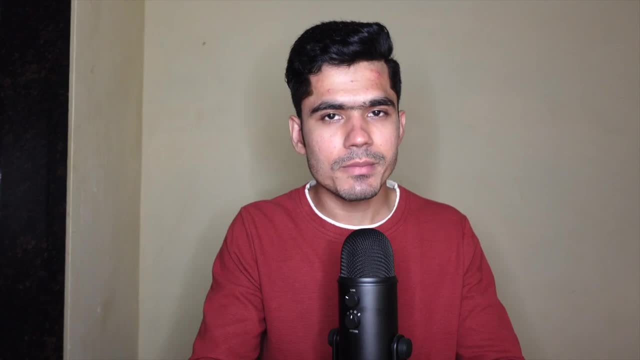 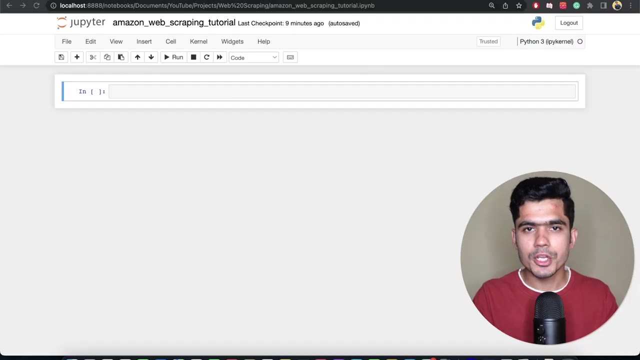 second thing, you need to install the Jupyter notebook. Just watch the first five minutes of the video and you will understand everything. Let's get started with the actual execution. So, considering you already installed Python and you already have the Jupyter notebook, that looks. 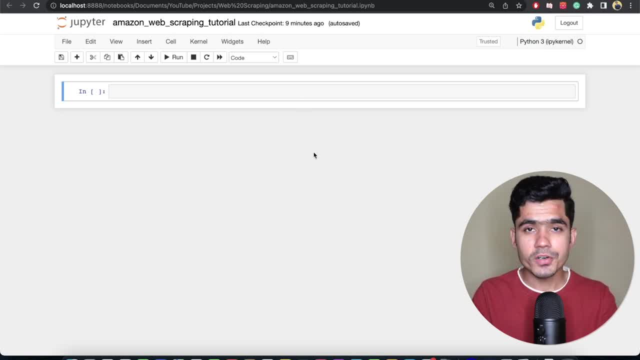 something like this: we will start writing our code Now. before writing our code, you need to install some of the packages that we will be using in this tutorial. First thing is Beautiful Soup. Beautiful Soup is a library that you can use to pass the HTML code. 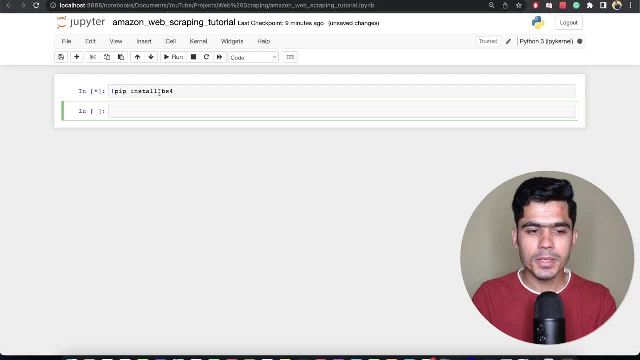 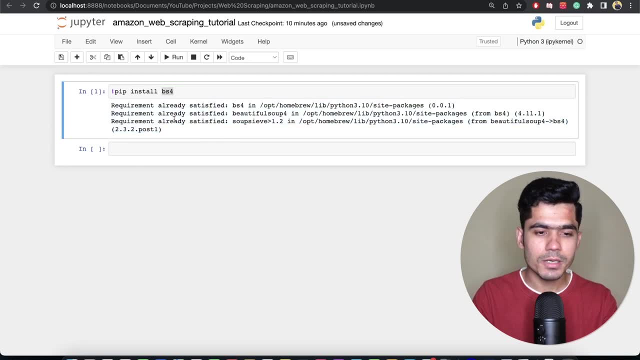 and find the elements inside it. So all you have to do is write pip, install bs4, and it will install Beautiful Soup in your PC. I already have it installed, so it is telling me that requirement already satisfied. But if you don't have it installed, it will install from the scratch. 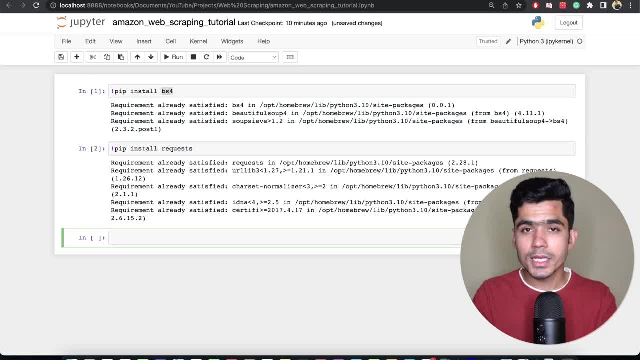 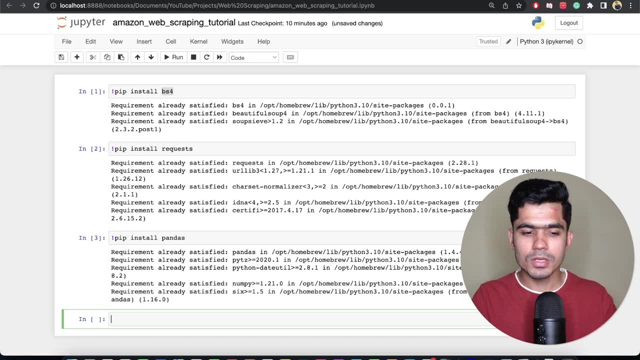 Second thing is you need to install request, because we will be sending requests from our local PC to Amazon website. Third thing we need to install is pandas, because when we scrape data from online, we need to convert it into the CSV format and we will be using pandas. 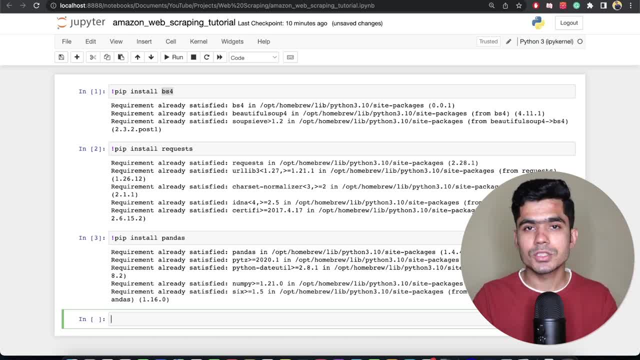 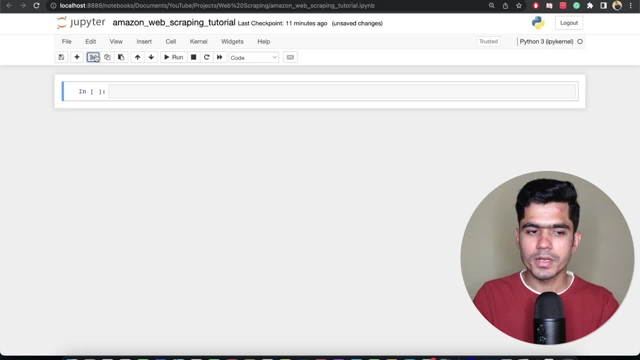 to convert those text data into proper data frame and then store it into CSV. So after you install all of these packages, you can clear it by clicking over here on the Caesar button and it will clear it. So now we will start executing our entire project. 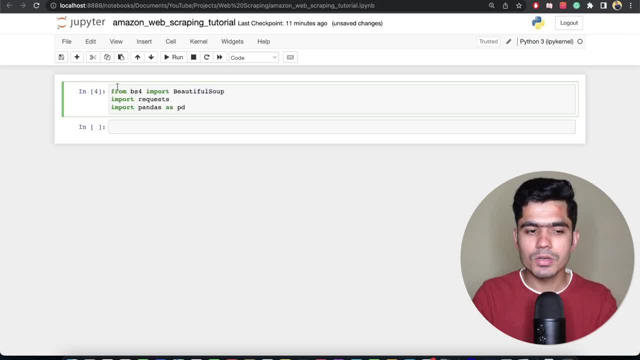 First thing is we need to import all of the packages that we so. this is how it looks like from BS for import Beautiful Soup, import request and import pandas. So if you understand the basics of Python, we are just importing packages. So now let's understand what we really want to do in this project. 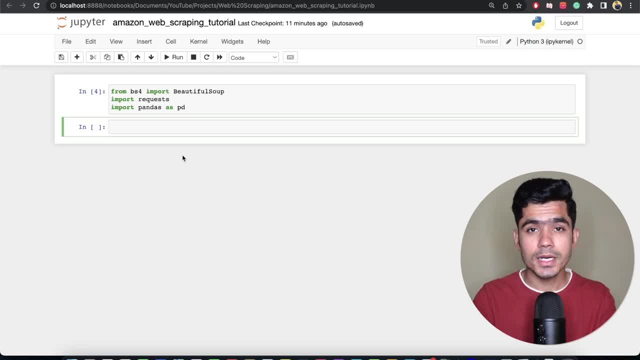 First we want to send the request from our local PC to Amazon website and get the HTML code so that we can get all the other information. So the first thing is we need to go on Amazon website. So I'm just going like amazoncom. 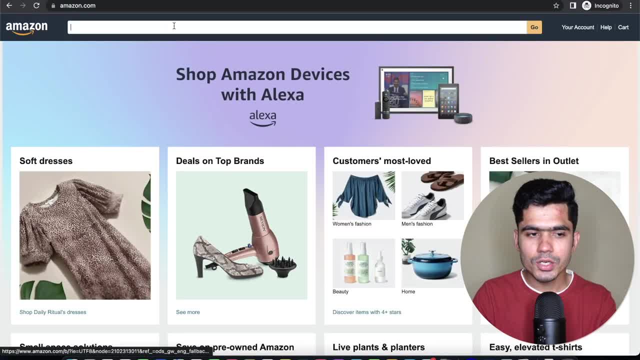 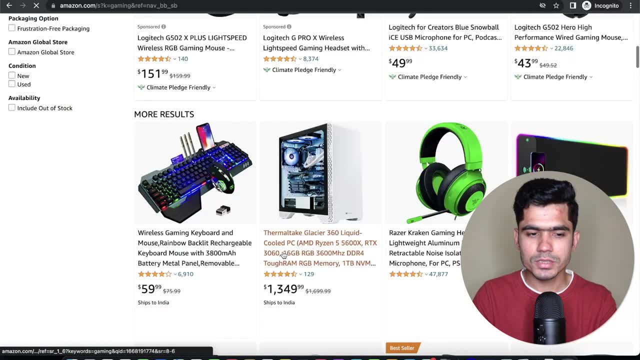 and this is what the Amazon website looks like. Now you can search anything over here, So I will search about, let's say, gaming. Okay, you can search whatever you want, And I see these products are on my site, So I will click on the screen Now if you want to understand the code. 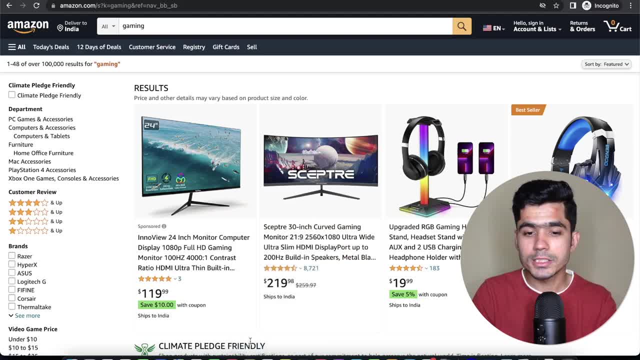 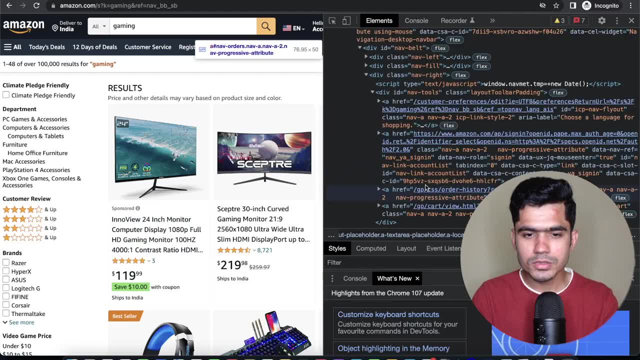 all you have to do is right click and click on inspect. on Windows it will be like inspect elements, so you just have to click it and you will see something like this on the side. So this is the code of this entire page. Now, this is what the code looks like. 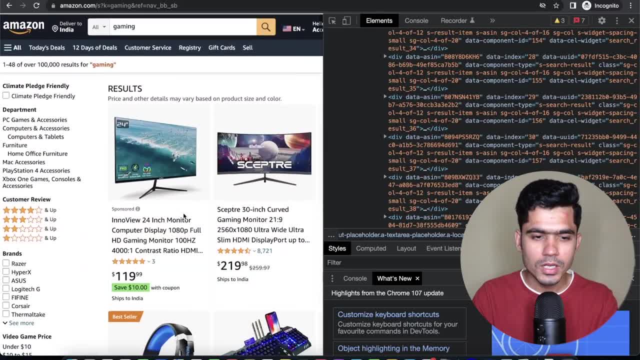 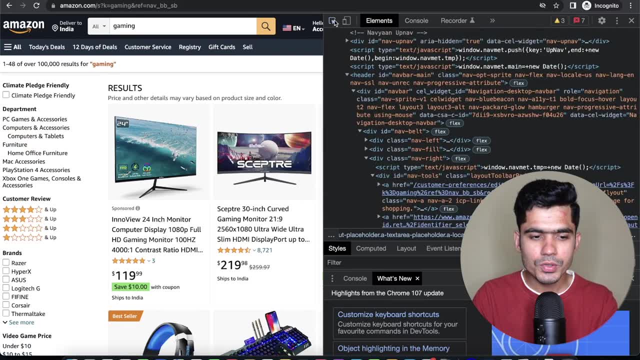 So this is the entire code of this page available on Amazon website. Now you can easily navigate to the page and find the elements on the website. All you have to do is click on this arrow. just click on it and you can move anywhere in the website. 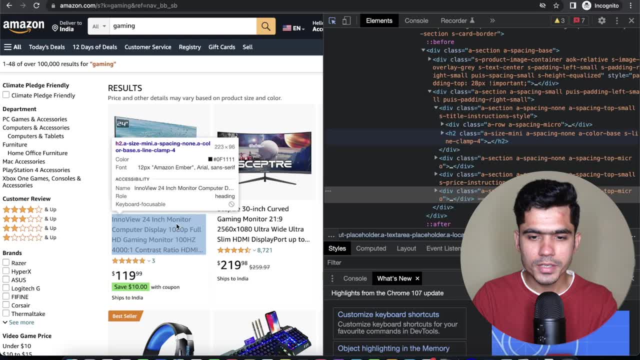 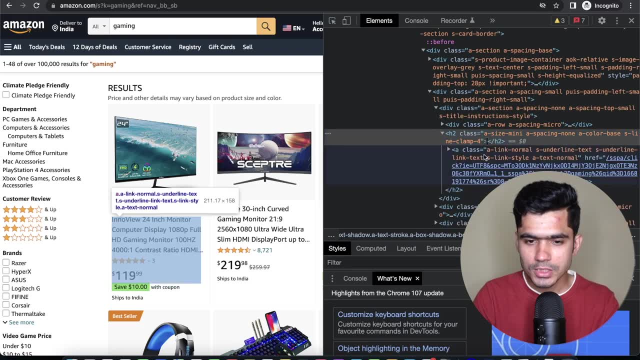 If I want to extract this title, you can click on it and it will directly take you to the actual HTML code that displays this title. So, as you can see over here, this is: this is h2 tag. h2 is the header tag. 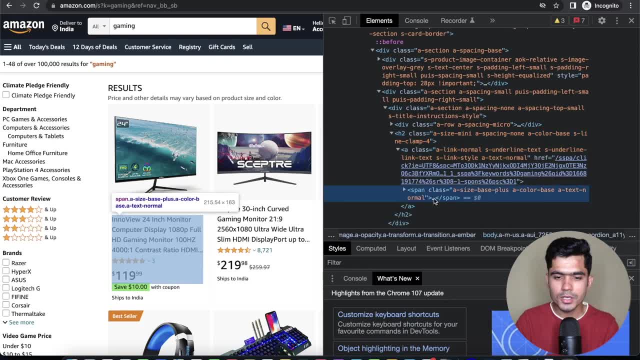 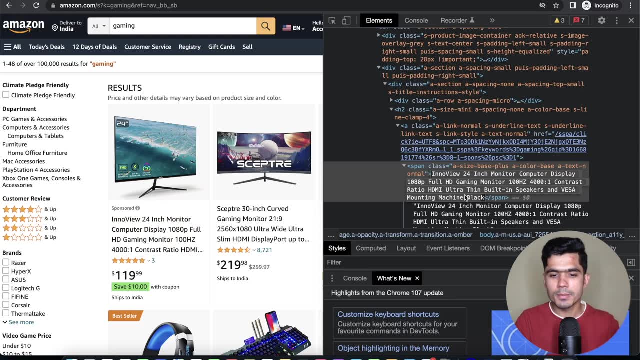 If you double click between these three dots, if you double click over here, you will find that this title that is being displayed over here, So this title is inside multiple tags. So this title is inside span. This is the class name, that is. 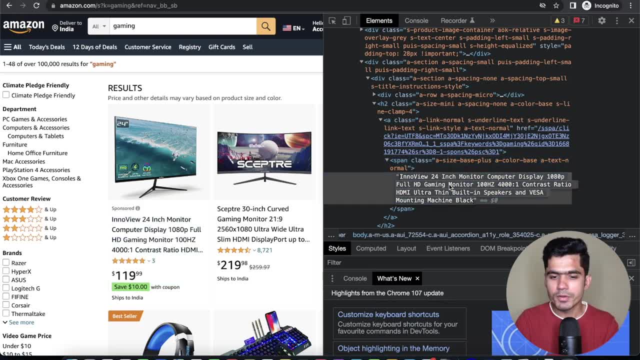 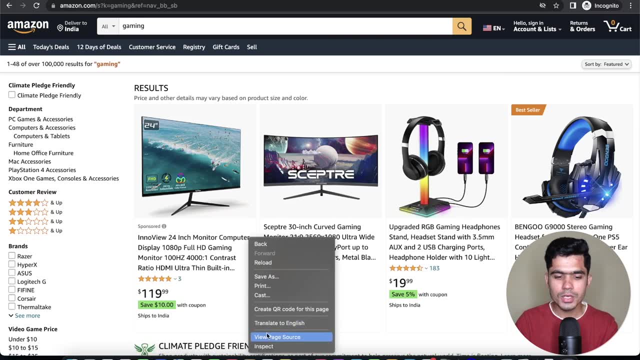 being used on this tag And this is the actual content that we want to extract. So this is how you understand the structure of the HTML. If you want to get the actual page so, you can just click on view page source and this will redirect you to the entire HTML code. 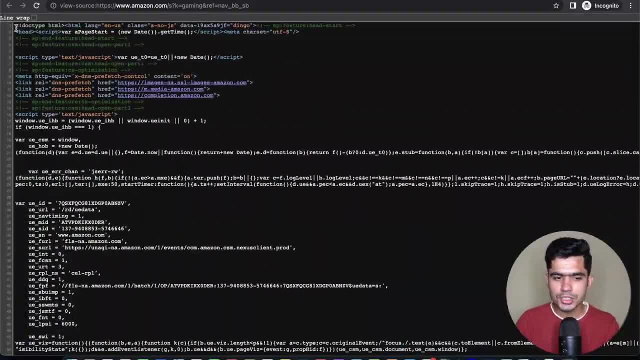 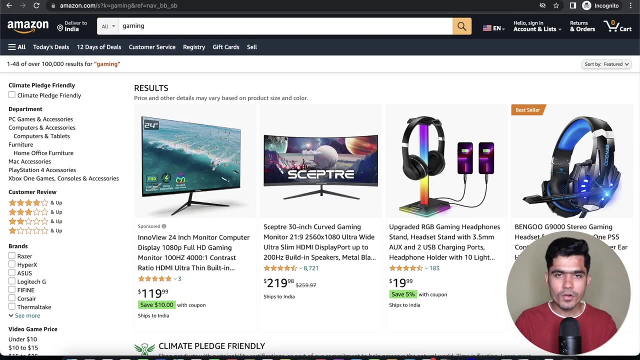 So what we really want is: we want to download this complete HTML document programmatically. So for that we will be sending requests from our Python code to the Amazon website, And for that we need to do two things. So let's extract the specific product information So you can. 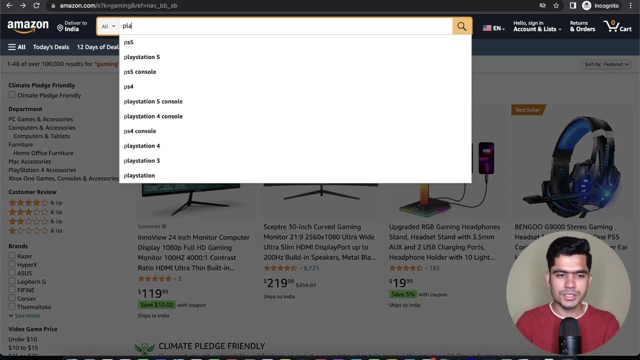 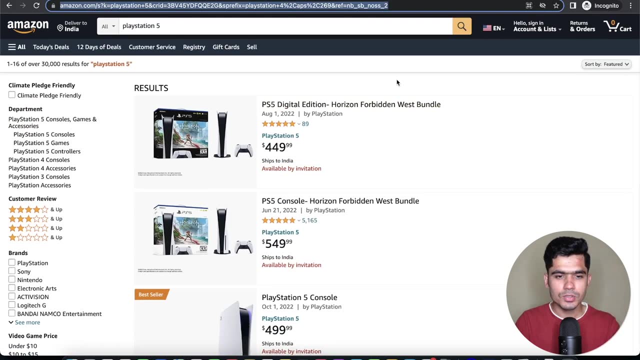 do whatever you want. You can do books, mobile phone. Let's do it PlayStation 4.. Okay, If you want to extract the information about PlayStation 4 or our code, we need two things. One is the URL. So let's just copy this URL and go inside our code- URL is equal to this- and just paste it as it is. 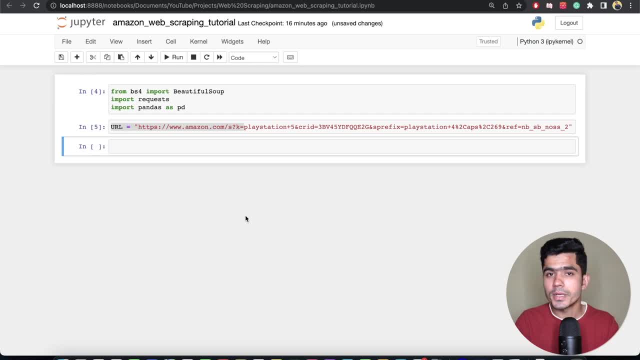 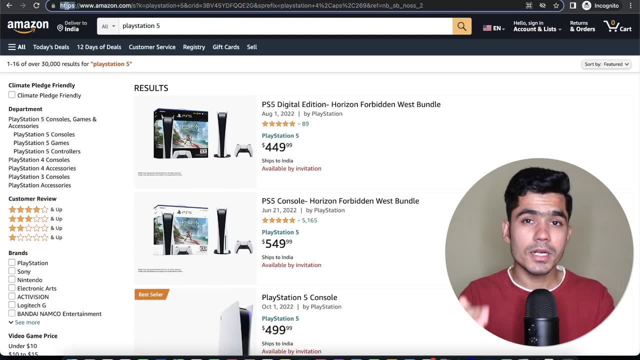 So we got the URL. Second thing we need to define is HTTP header. So whenever we visit any website on the internet, you send HTTP request to it. HTTP request contains a lot of different things, and one of the most important thing in that is user agent. User agent tells that you are trying to. 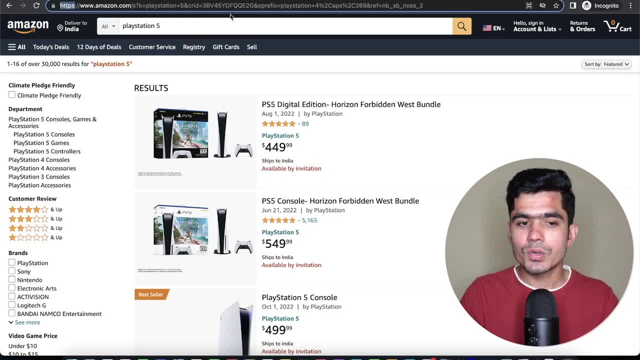 access this website and you are a genuine user by identifying your browser information and some of the other information required to access the website. This is just basic. If you want to understand more technicalities of user agent, you can go and read more about it, but you need to get. 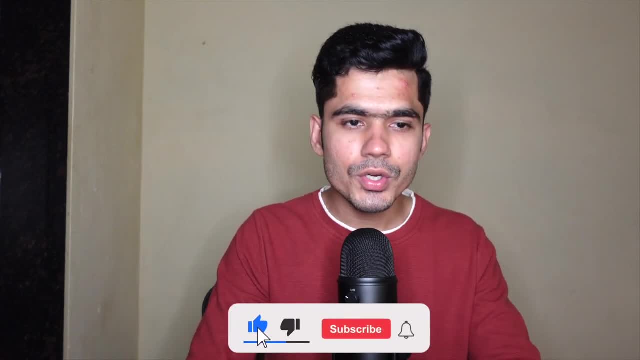 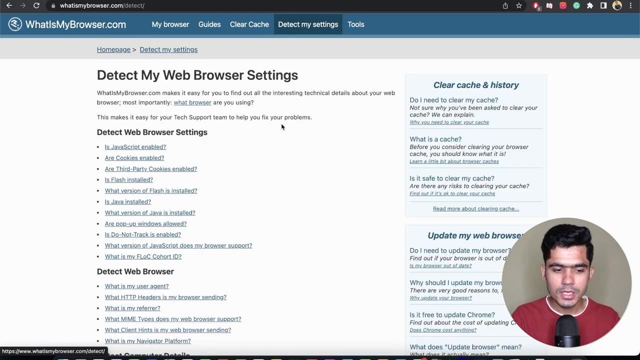 your own user agent. And how do you get it? You can go to whatismybrowsercom. You have to click on detect my settings and you will see that. you have to go to whatismybrowsercom and you have to detect my settings and just click on what is my user agent. You will see something like this All. 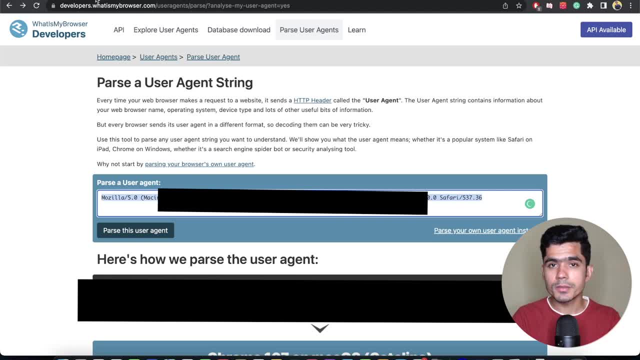 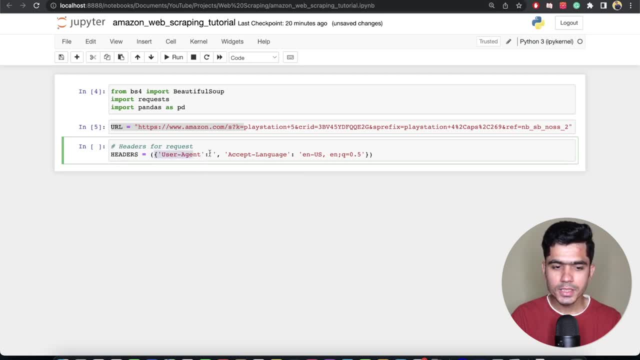 you have to do is copy this user agent. You might have your own user agent based on your browser- and paste your user agent over here. So we are defining header inside the user agent, We will paste our user agent and we are also defining the language. except language is English because 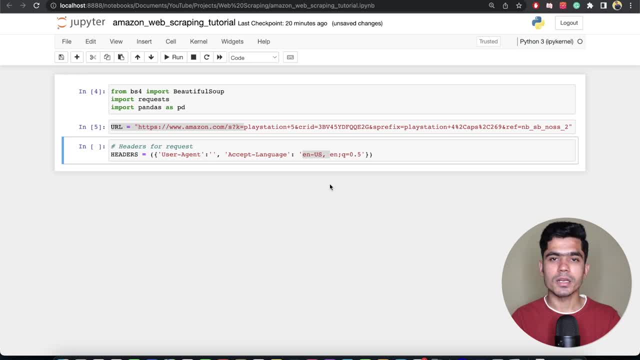 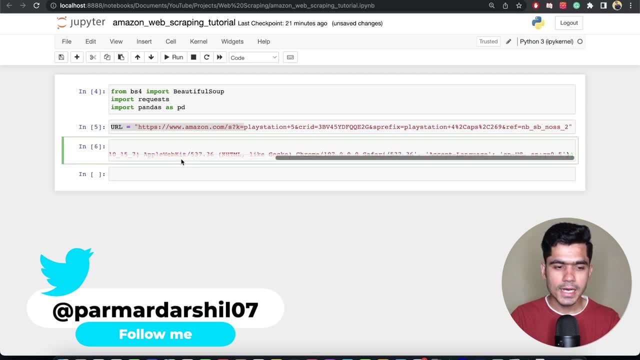 inside the request. we want to tell Amazon that we want everything in English language. So all you have to do is paste your user agent over here and just run it. So you just defined your header and URL and now we will be making requests. So let's go ahead and run it. So you just defined your header and URL and now we will be making. 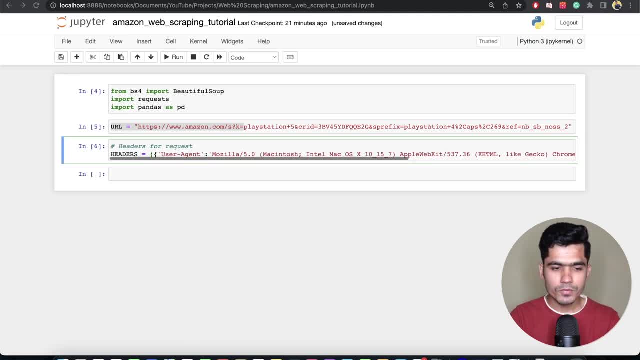 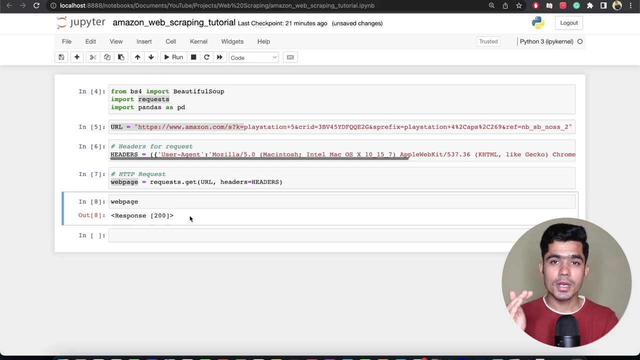 requests to the Amazon website. So for that, to make the request, we will be using request package get. We will pass our URL and we will pass our headers and just run this. Now all you have to do is check if you got the response 200.. If you got the response 200, that means your HTTP request was. 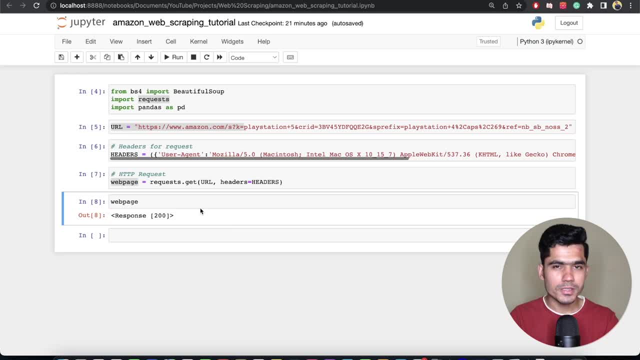 successful. If you are getting 503 error, then you can try after some time. even if it doesn't work, then you can try some other user agent. You can find it online, or even if that doesn't work, then Amazonin or Amazonuk based on your country, and it should work okay. So if you get the 200, 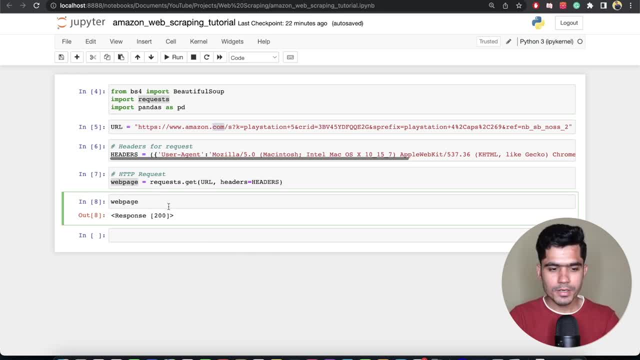 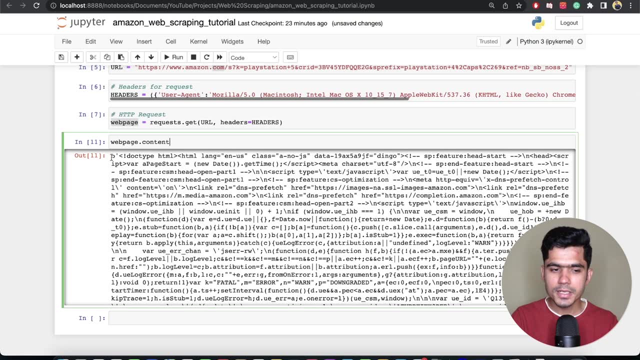 response, then you are good. Let's print content from this web page and you will see the entire HTML document that we got. So currently, this request is returning this HTML document into bytes format. So if you just write type, you will see this is in the byte format We want to. 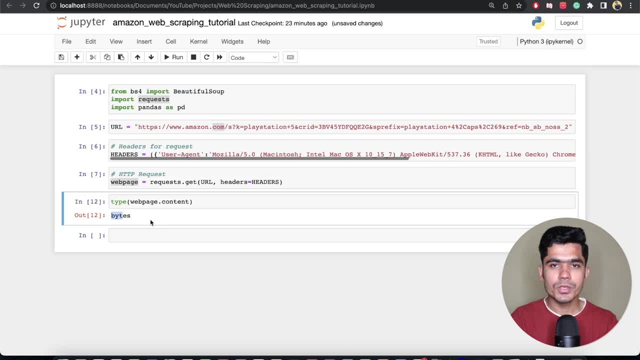 convert this into proper HTML format, and for that we will be using beautiful soup. This is very. all you have to do is use the beautiful soup function that we imported, Send your web content and pass it into the HTML format. If you do that, and if you just print soup, you will see proper. 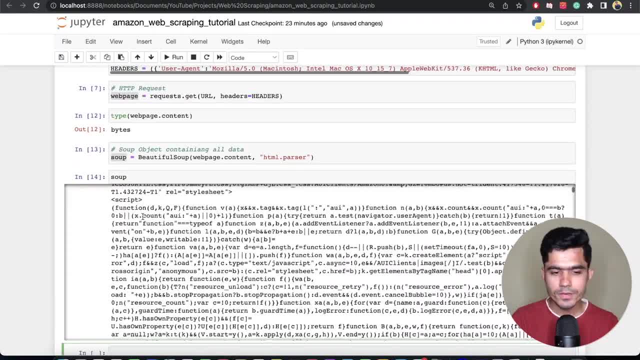 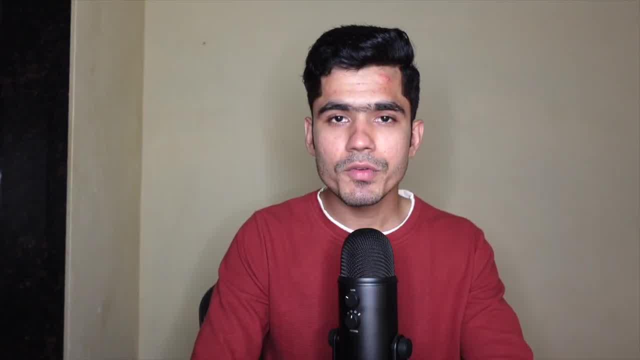 HTML document converted into HTML file, So you will see a lot of different things. We don't want to get into everything right now. We will go step by step. So we were able to extract our HTML document. Now what we want to do? we want to find different links available on that page. So what? 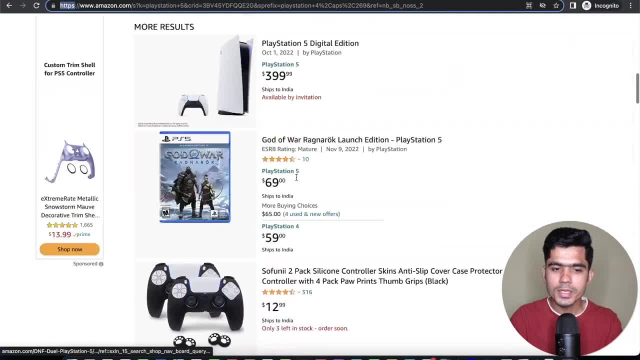 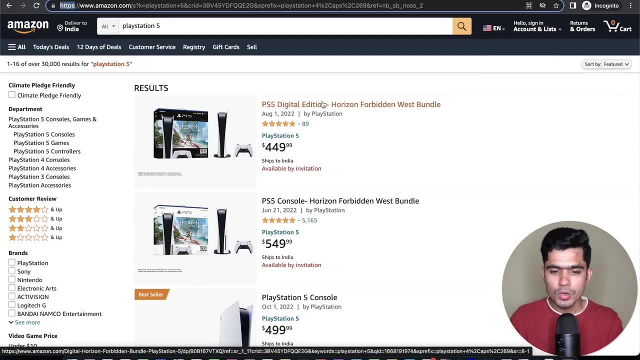 we want to do is we want to go through this entire page and we want to get the product links so that we can iterate on each and every link and go and extract information from the pages. So for that you just have to go to inspect element and we want to find the links. 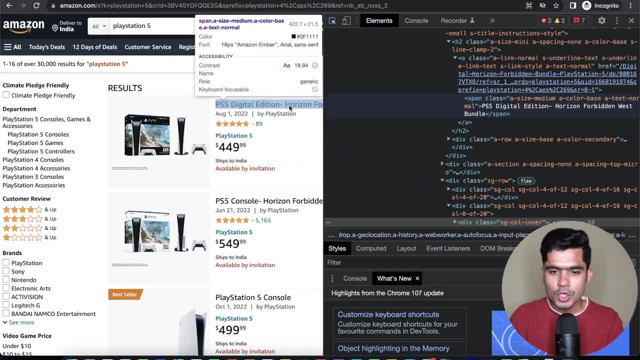 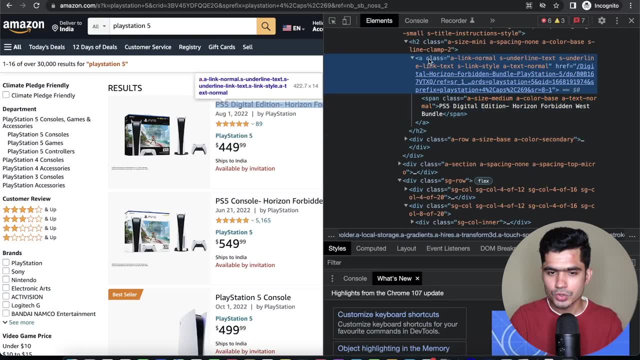 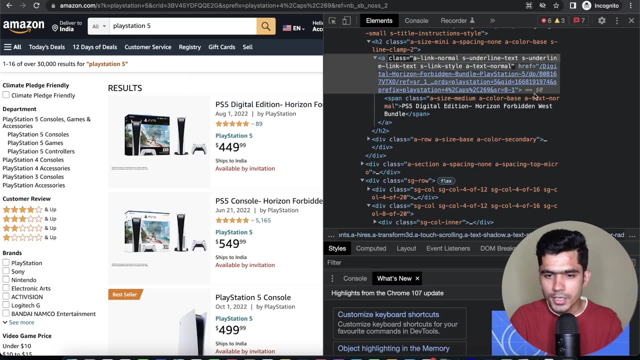 So if you have basic understanding of HTML, you will understand that all of the links are written inside the a tag that is called as the anchor tag. So over here we are also seeing that a class and this is the class information, and you will find some kind of links. 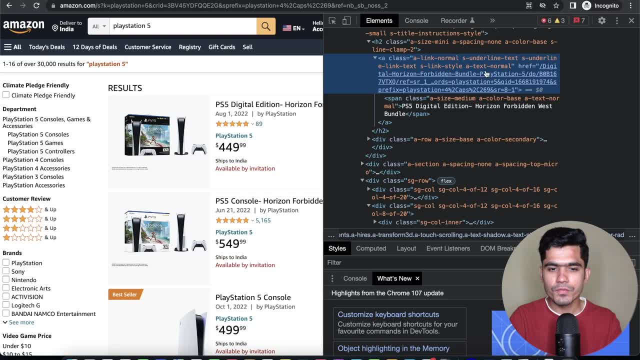 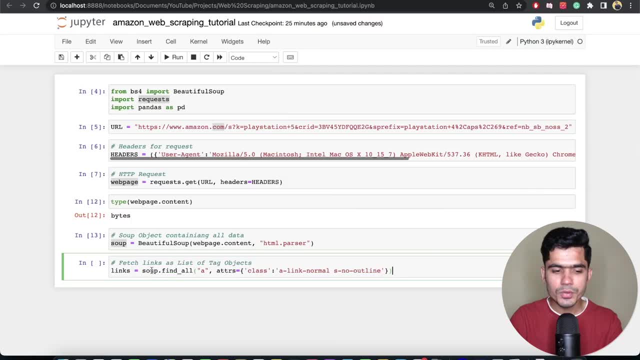 href element. So for that we need to find this a tag with the class name like this: So let's just try to do this practically to understand what is happening. So all you have to do is there is a. so there is a function available inside the beautiful soup. this is find all, Find all, all of the a tags. 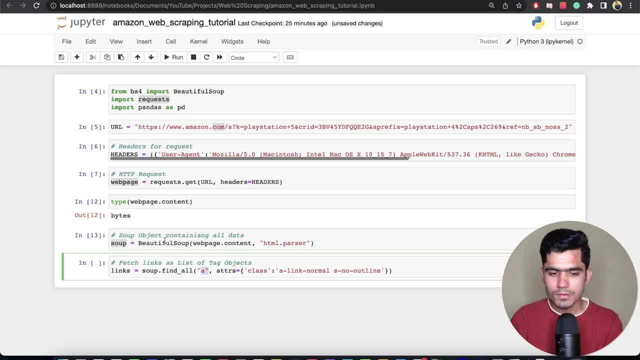 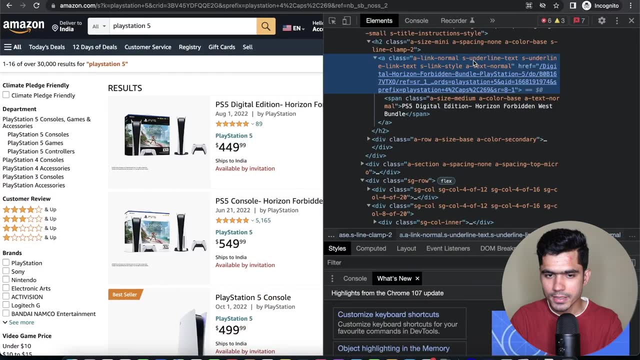 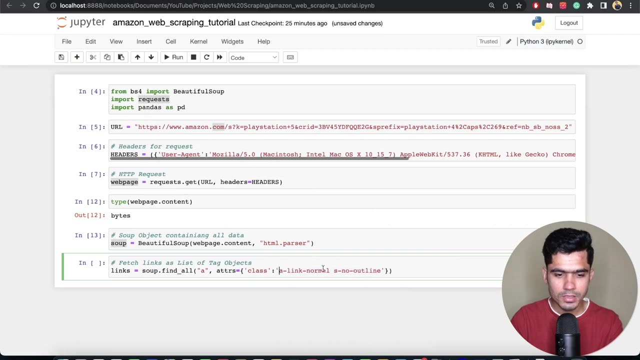 available inside our page that we just extracted, where the class name is. whatever the class name there was inside this anchor tag, You can copy this entire text, okay, and just paste it on your code. let me just copy and paste it and let's see if we get something. yes, and just run it. 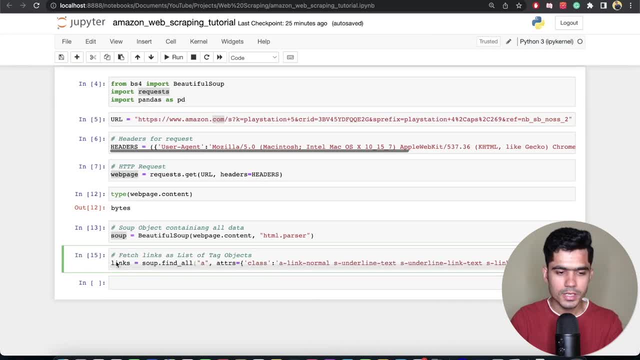 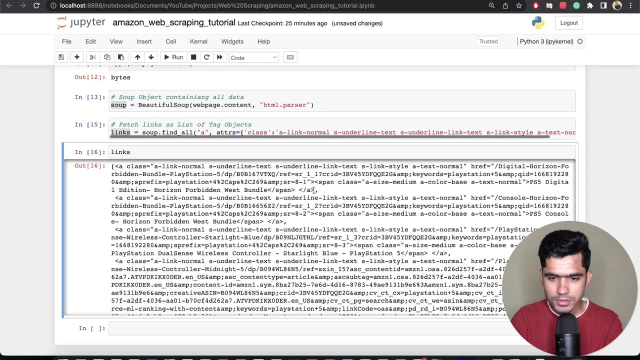 and let's see if we got the links. copy links, paste it over here and you will see we got the list of different links from that page. So let's say this is digital horizon something. let's just say the ps5 digital first edition horizon forbidden west bundle. okay, if we go to our amazon page and that's. 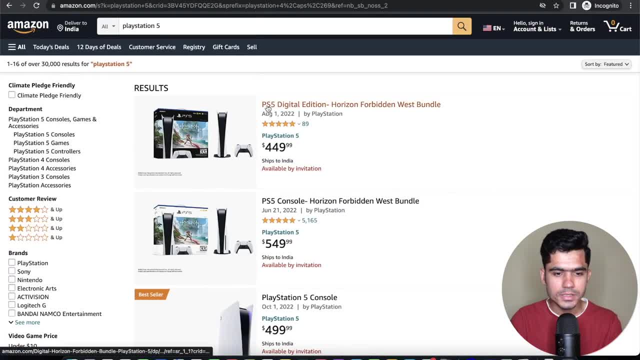 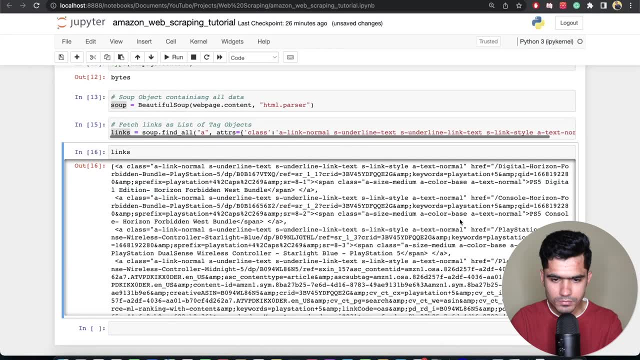 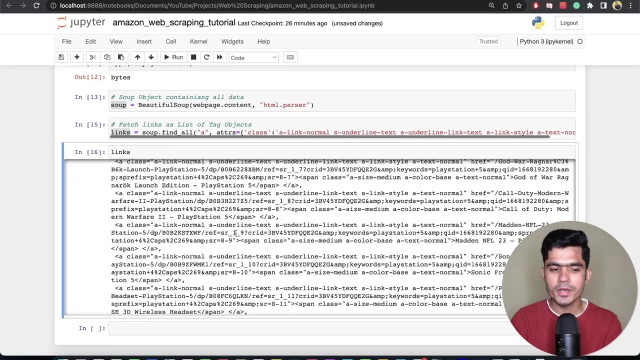 should be our first product. if you see the second product, ps5 console, horizon- bundle west, bundle- okay, ps5 console. let's start with the ps5 console. where is that? yeah, ps5 console, horizon forbidden. okay, so we were able to extract all of the a tags. if we did the find, all that means we were able to. 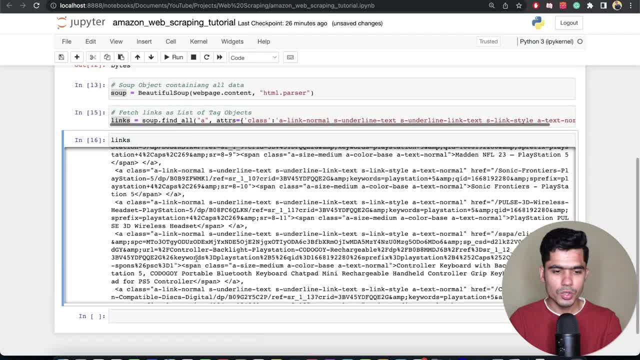 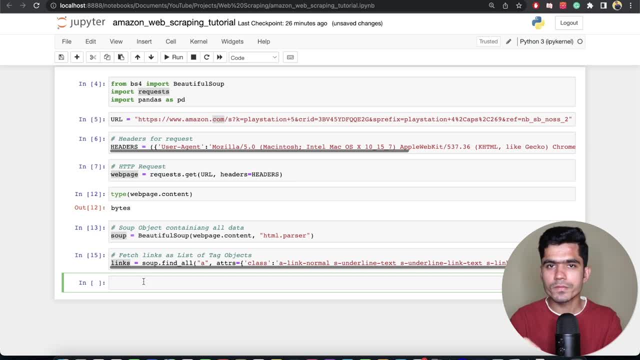 get all of the anchor tags from that particular page, so we were able to extract the links now. for now we will just do it for the one link and try to extract all of the information, and after that we will just loop through each and every link and build the proper. 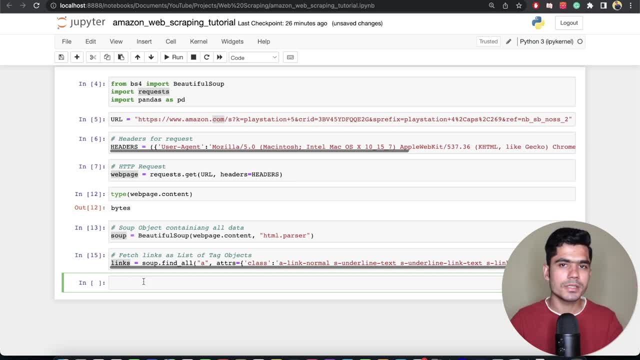 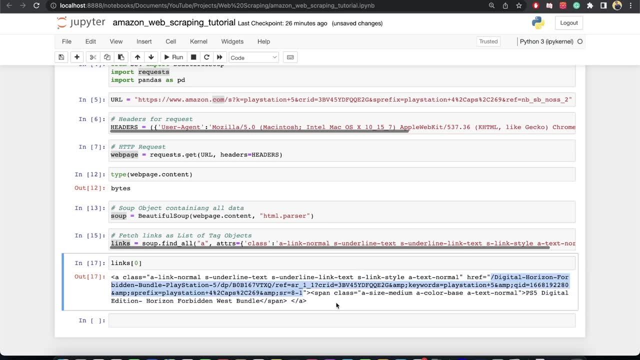 function so that we will get everything automatically inside the pandas data frame. to extract one link, all you have to do is links okay and slice this: uh, zero, so we just get one link. so now what we want to do? we need to visit this products page, so so we want to visit over. 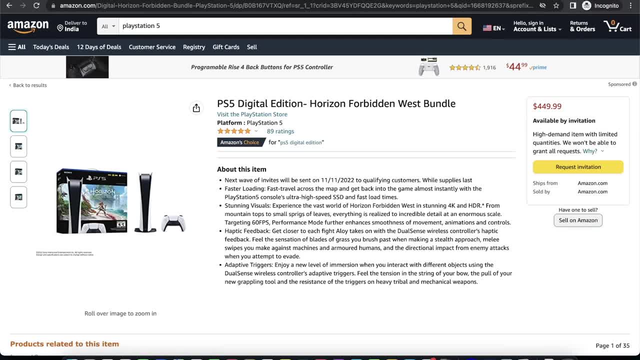 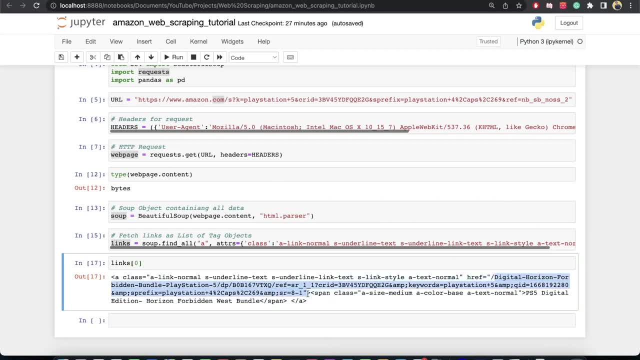 here and for that we need to build the proper link. so, as you can see, over here we just we are just getting half link over here. we need to append some things over here. so first of all, let's extract the a tag. all you have to write is dot get h r e f- this is same as href- and just run it and you. 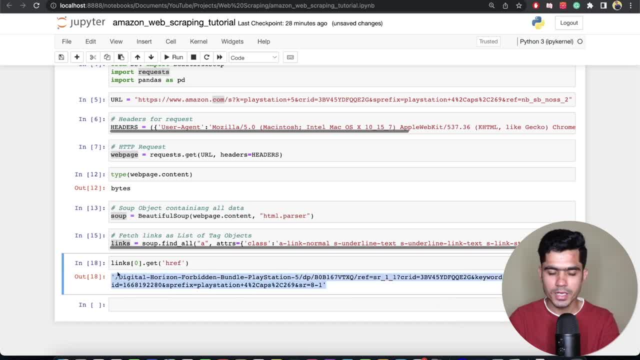 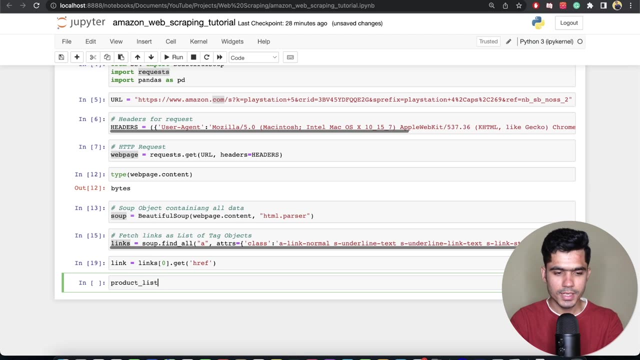 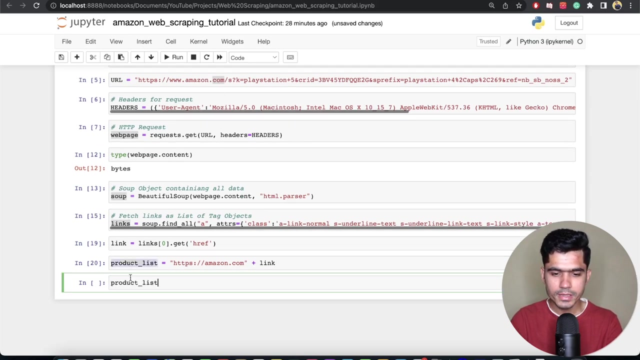 are able to extract the actual link. this get function, href and you will be able to get the link. now let's just store this link into uh, link, okay, link variable, and for this we will append product link is equal to https, slash, slash, amazon, amazoncom. okay, plus link. okay, if i do this, if i run this, i will get the entire link. 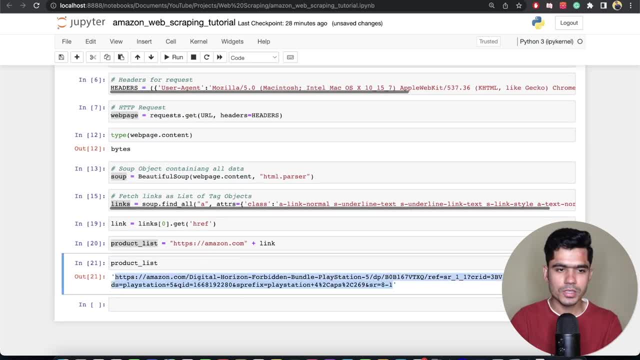 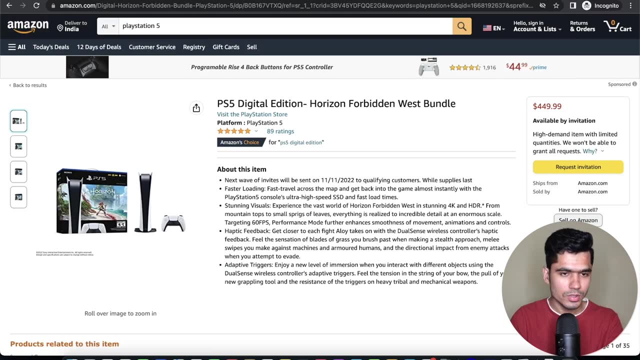 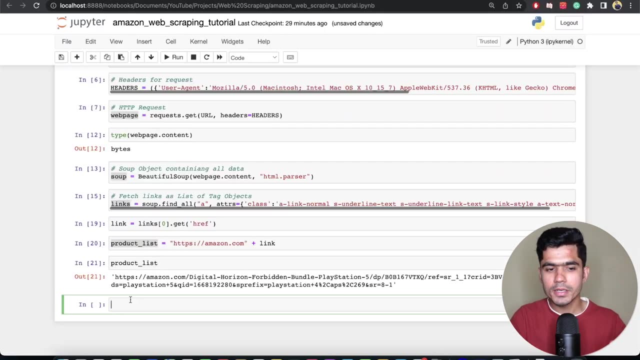 you can copy this link and you can paste it on your browser to see if it works or not. and it is taking us to the same page. uh, that we went earlier, so our link is working. we were able to successfully get the right link in our program. now again, we want to repeat the same process. we. 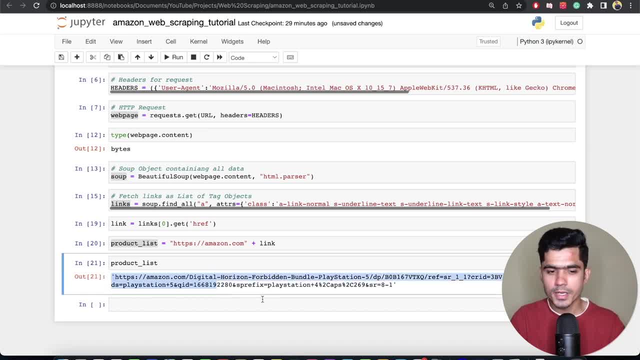 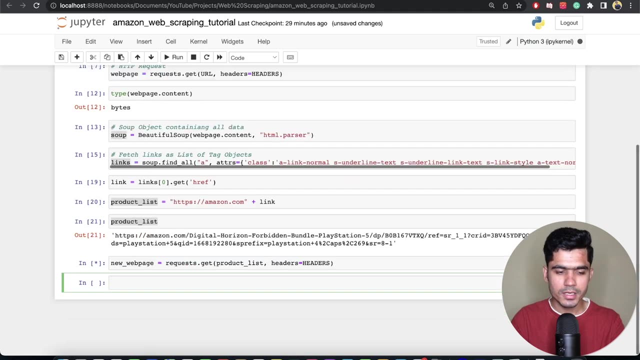 need to make requests to this page to get the html document and then pass that page into html format. so we'll be doing the same thing. just copy this. just write new web page. your url is the product list over here. headers are the same. just run it. just check if your request got successful. 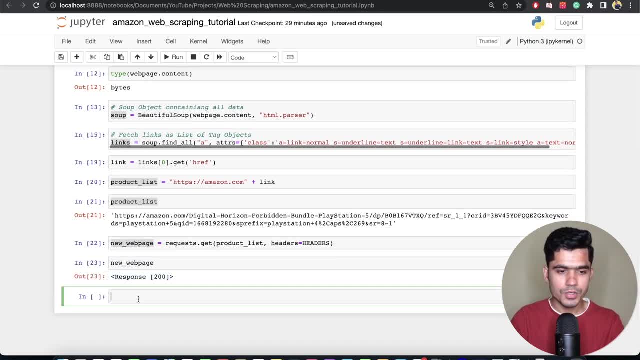 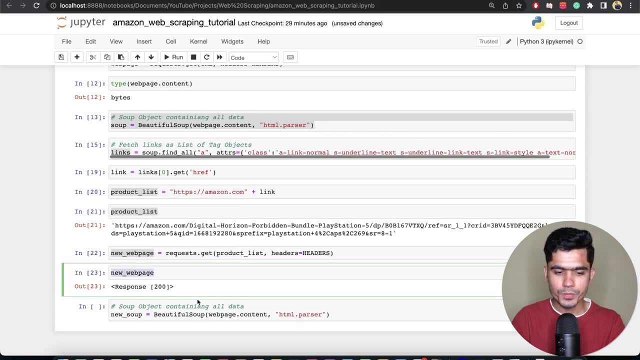 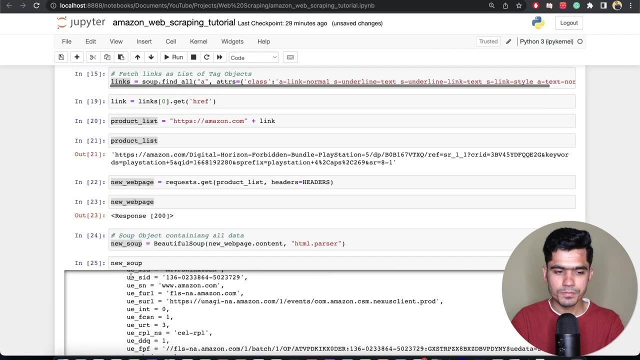 200. that means your request was successful, and then you need to pass this: just write like new soup web page to new page content html parser and pass this html over here, so you'll be able to get this entire function. okay, so this is a bit straightforward. this is what we did initially, what we are really. 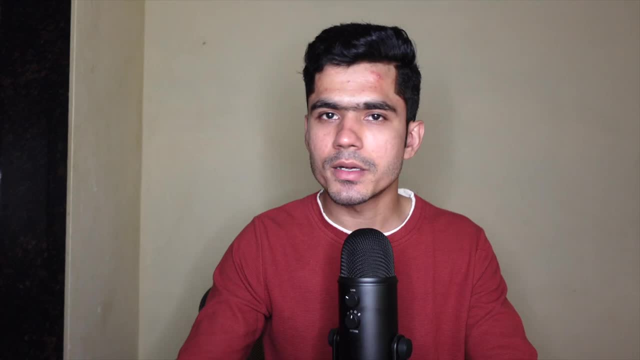 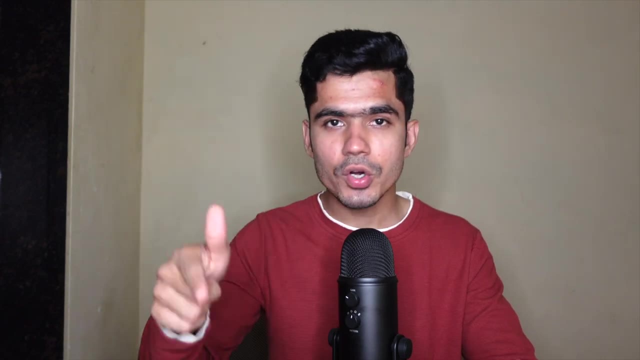 trying to do over here is that we're just going step by step to understand the entire process and how to get the element from one single page. once we are able to get that, then we can easily loop through this, all of these pages, and get the right information. then the next thing we need to do we 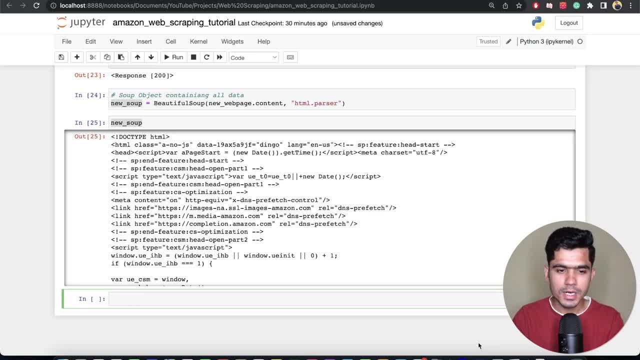 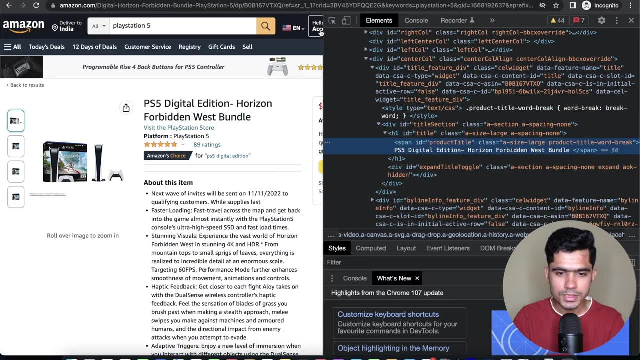 need to get some of the information from these pages. so let's start. let's go ahead and start. let's click right, click inspect element. let's say, if you want to extract the title, okay, click on this arrow. click on this title and you will see span id is equal to product title. so so all. 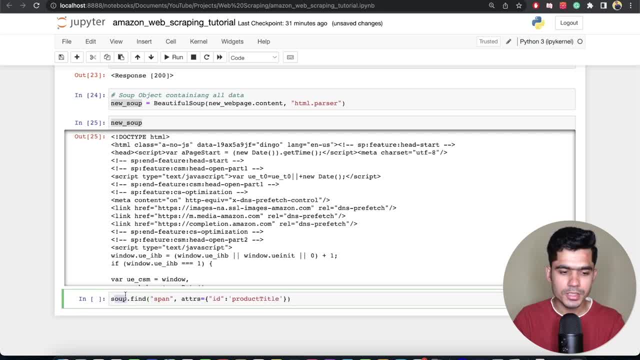 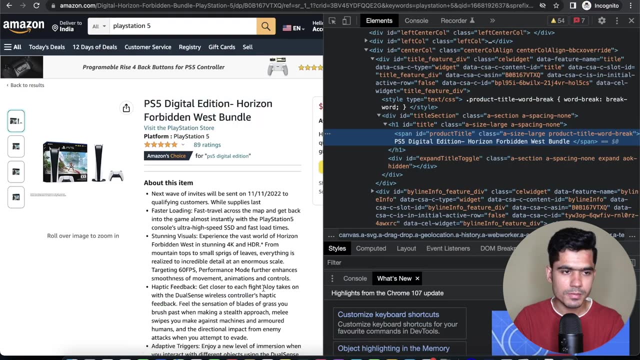 you have to do is write something like this over here. let's change it to the soup, new soup find. span id is product title, so attributes are id and it is product title. this is same as what we are seeing over here: span id, product title. and if you run that, let me just minimize this. 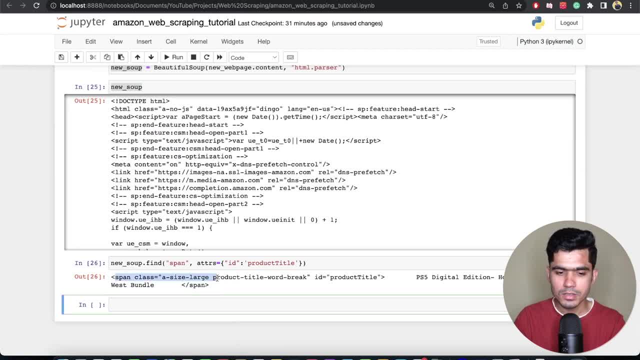 you will be able to see this entire html code extracted. now, to get the content, just the text, out of it, all you have to do is write text. you will see something like this: but we are seeing some of the white spaces over here, uh, and over here, and to remove those white spaces, you just 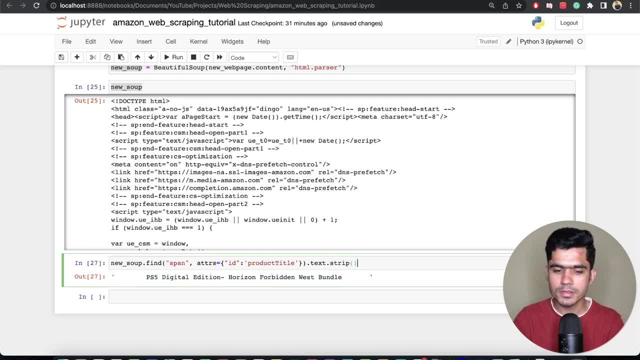 have to write strip. this is a function available inside the python and it will remove all of the white spaces from left and right. so we were able to extract the proper title. uh, over here. uh, let's, let's look at some of the other information that we want to extract. so let's say if we want to. 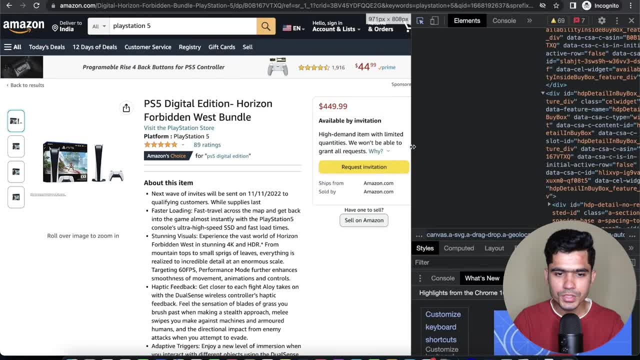 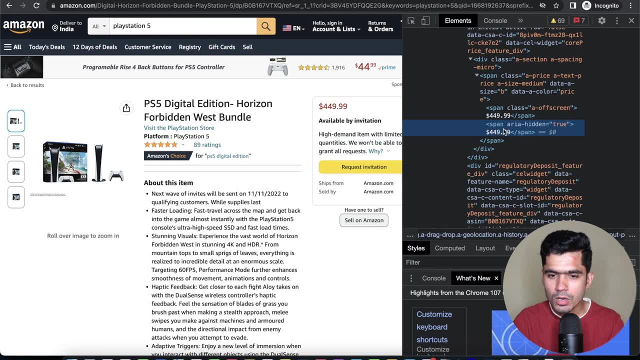 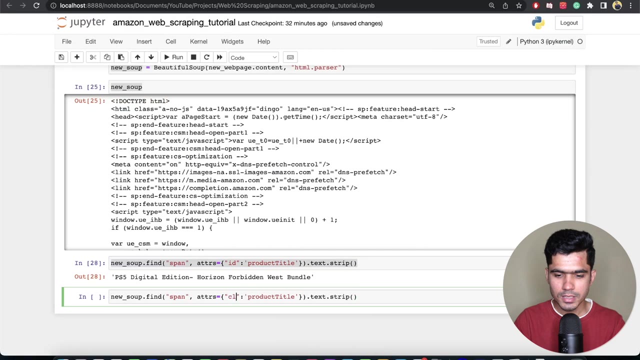 extract. let me just put it over here. let's say, if you want to extract price, okay, click over here. you will find this span, class or price tag, size, medium, okay. so let me just- so let's just go back- copy this span. this is class and inside the class we have. 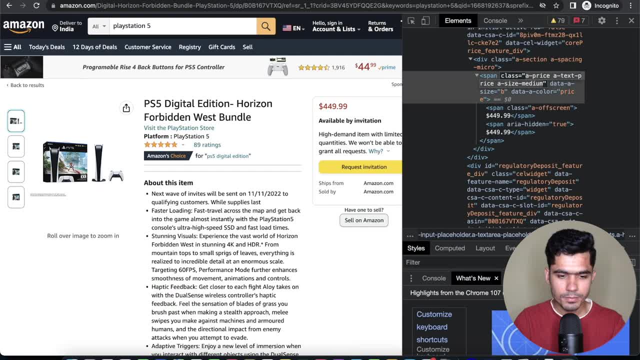 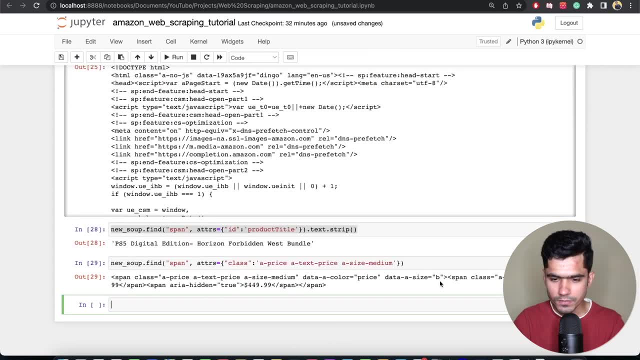 this class. just copy it as it is, paste it over here, remove this for now and just run it. so we were able to get this information. now, as you can see, we are getting this pan. inside this pan there is one more span that displays one price- the off-screen price- and inside this pan we have one more span. so if we do the 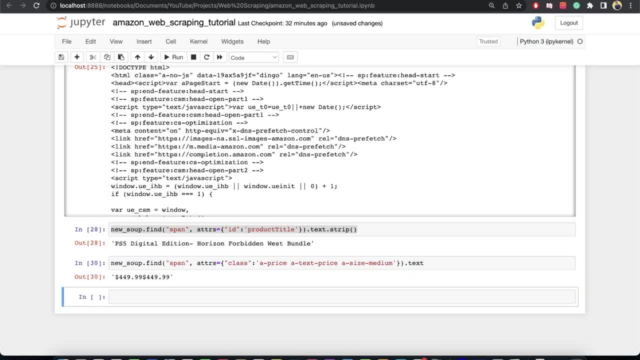 text over here, we will get some something, some duplicates, so so. so if we do this, if we do this, we are getting duplicates. so to handle this situation, what we can do is dot find. you can also do find on top of it. span attributes is equal to class colon, and let's just get the first one. 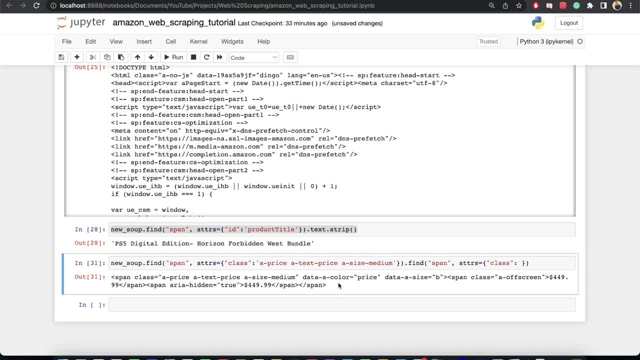 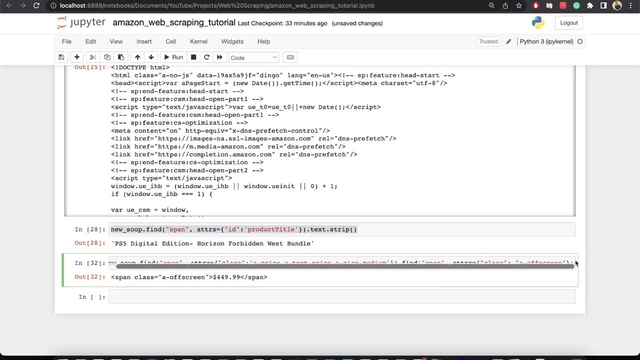 oh, let's just get, let's just, let's just get the first one off-screen, and if you do this you will just get first thing. so now you can do dot text to extract the price. how easy that is. so we were, so we were able to extract the. 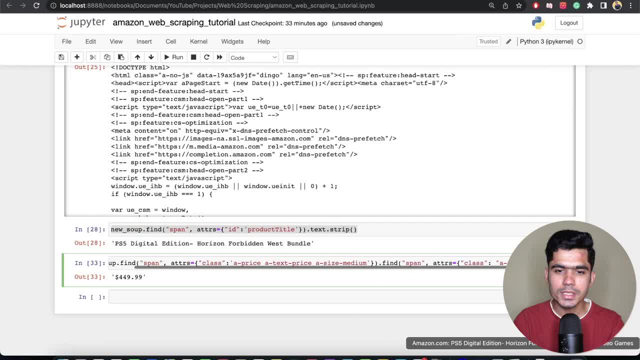 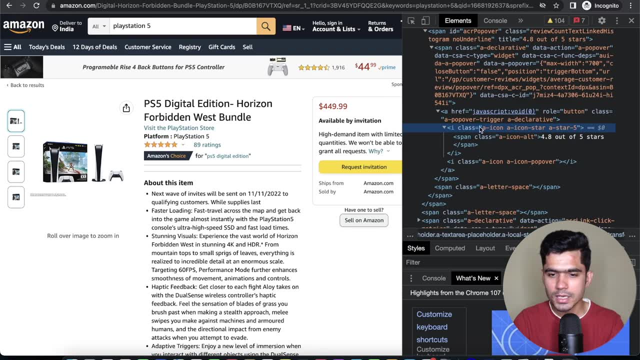 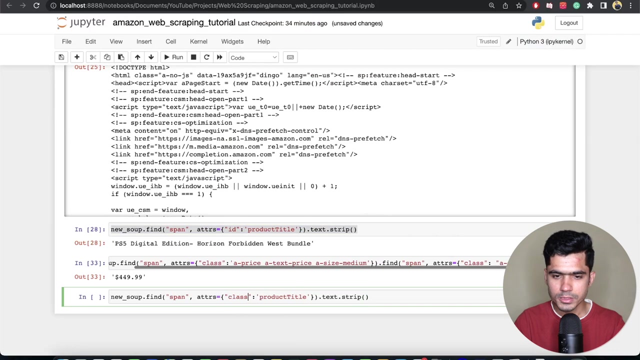 price like this. then again, you, if you want to extract some other information, let's say if you want to extract this ratings, okay, so, so over here. so over here, as you can see, we have span class, a icon alt. okay, so we have to repeat the things over here. just minimize this. let me just copy this span class, was it? 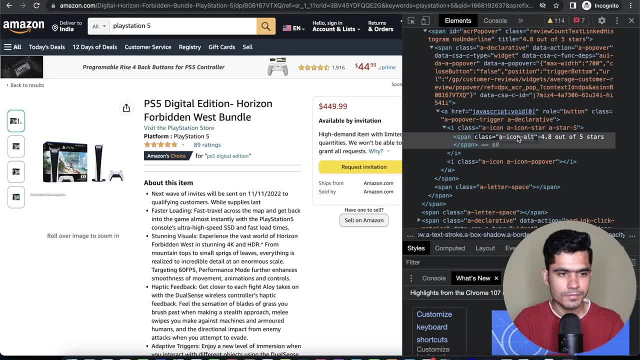 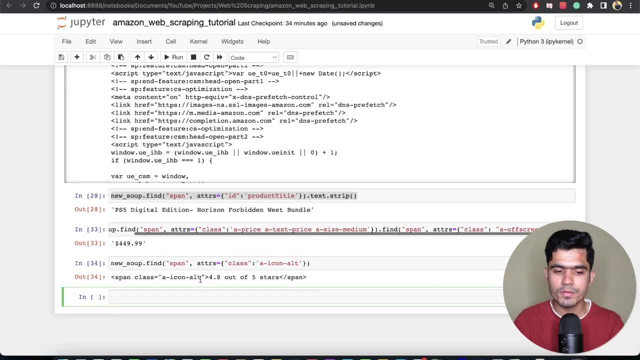 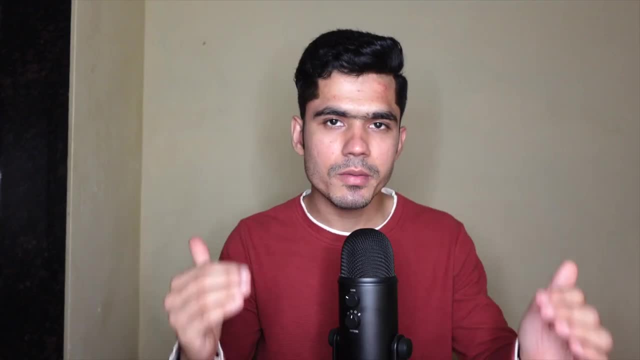 span- yeah, span class a icon alt. let's just remove this. hopefully this works. so we were able to extract 4.8 out of 5 stars. you can do text and you will get the actual thing. so you understand the process. all you have to do is whatever. 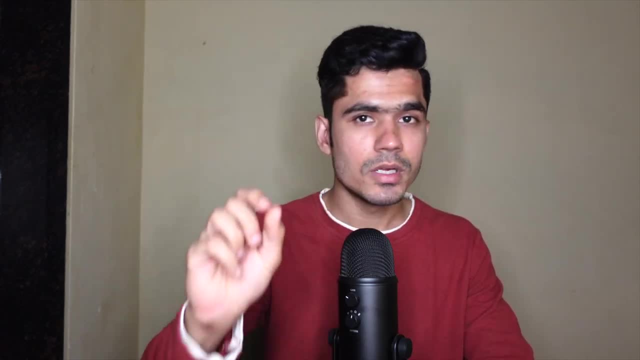 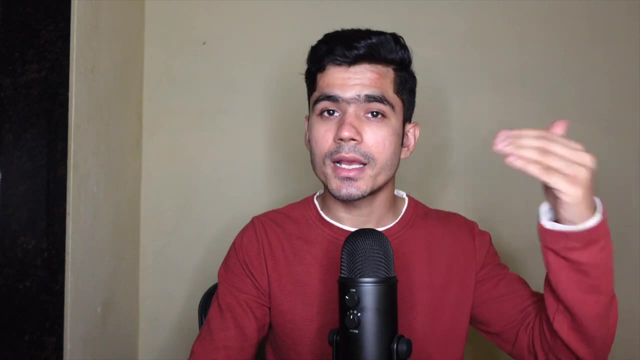 the element we want to extract. we want to find the tag name, the attributes, like it can be ID class and copy the right attribute and just put it over here. if it is nested, then what you can do: find inside that element and find the right element, just like we did for the price. so this is step-by-step approach. so we 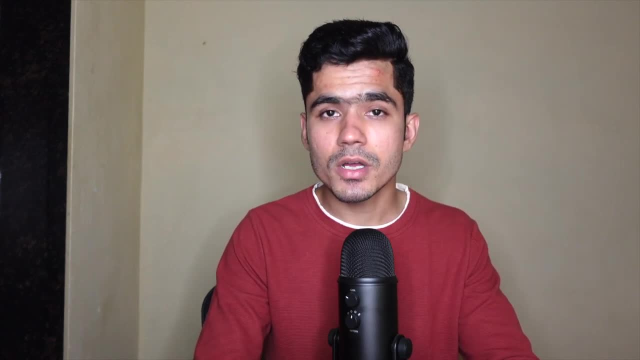 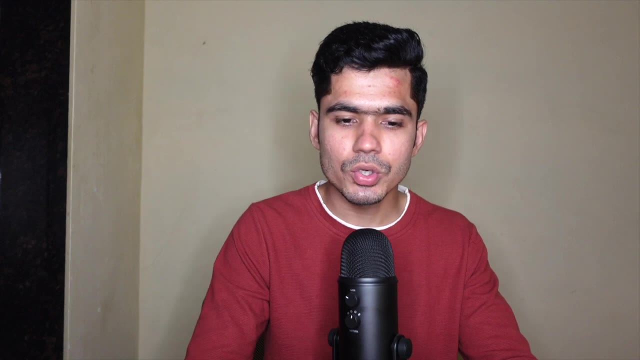 were able to extract, like some of this element. now, these structures might be different according to your region. so Amazon keeps changing these things to you know. protect their website from this web scraping and all of the other things. so if these, these exact text, doesn't work, try to go and 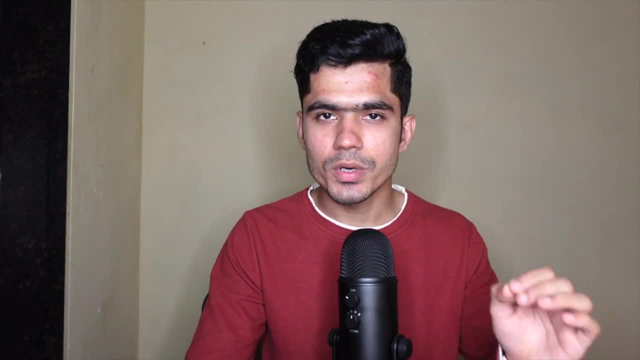 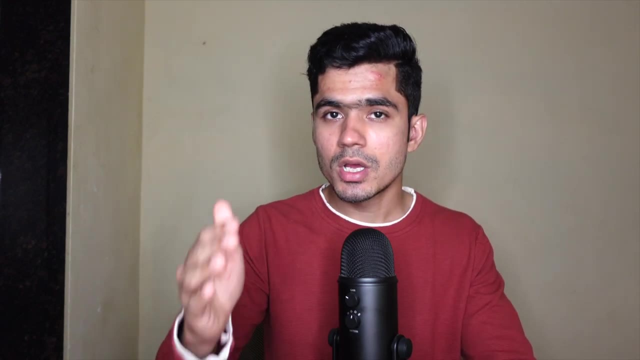 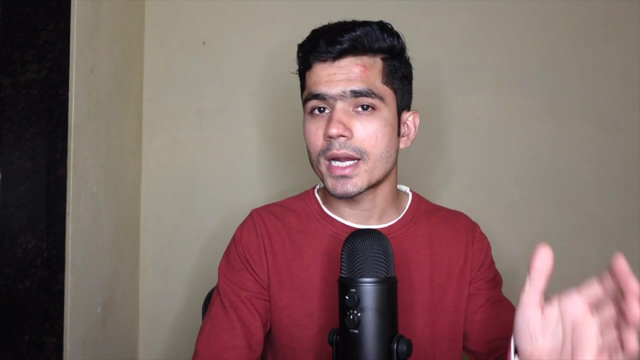 check inside the code and see what is the actual code over there and modify your code accordingly. I'm not 100% sure that this one code will work. you have to understand a structure and then put the right information on your code, so this was just a procedure way of doing it. now I'll just show you one of the code that 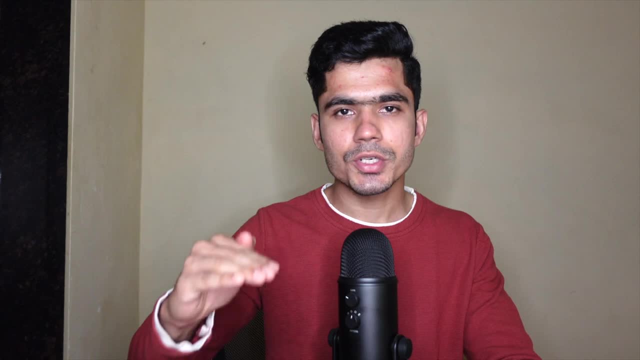 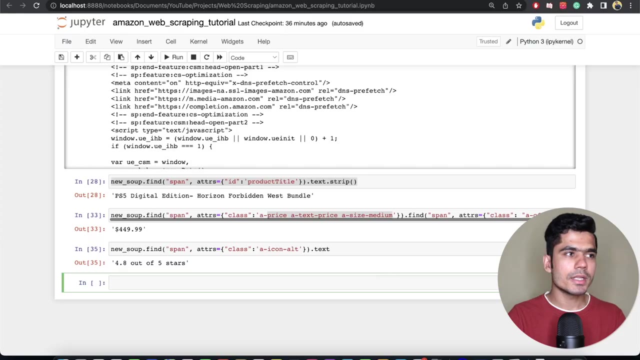 I've written and explain you step by step how it works, because you understood the fundamental of how to extract data from Amazon website. now you will understand how to put everything together and make it work. so I've already done that, so you don't have to spend your time doing one thing again and again. so over here, again we are. 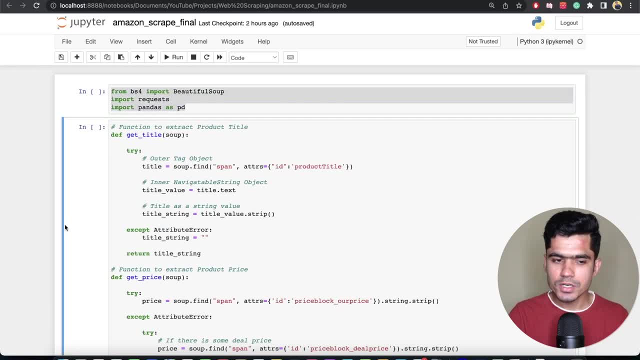 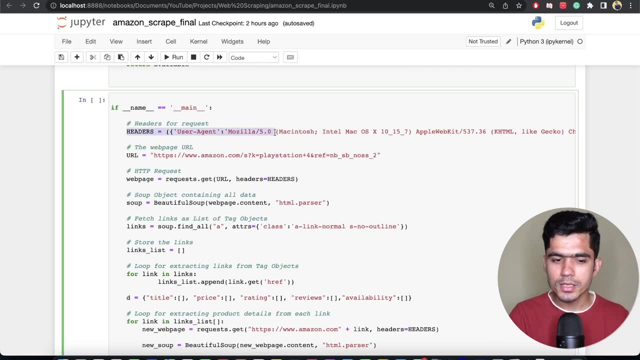 starting with importing our packages, then I will come back to these functions. let's understand the basic things of our code. first thing is the header that we defined. then the second is the URL- now URL. you can replace whatever you want. then what you are doing: we are doing the same, sending the request to the Amazon. 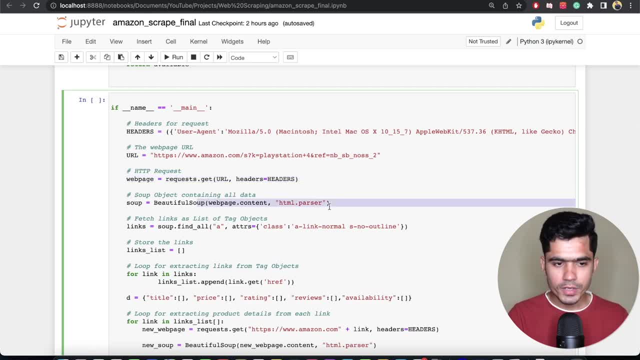 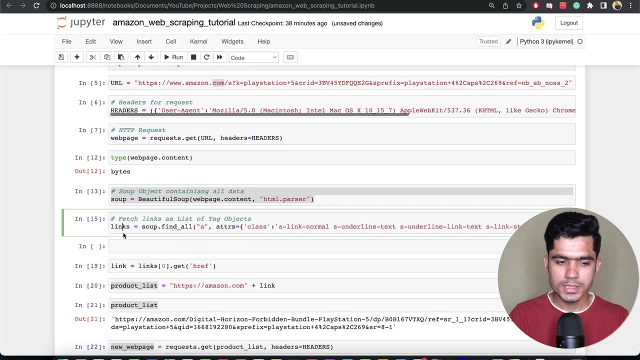 website, then parsing it into the beautiful soup. so, whatever we did in our code- yes, following the same things, and what we are doing is finding all of the anchor tags- um same we did over here, just like this, that this will basically return all of the links. uh, let me just show you again so that you guys can remember it. so all. 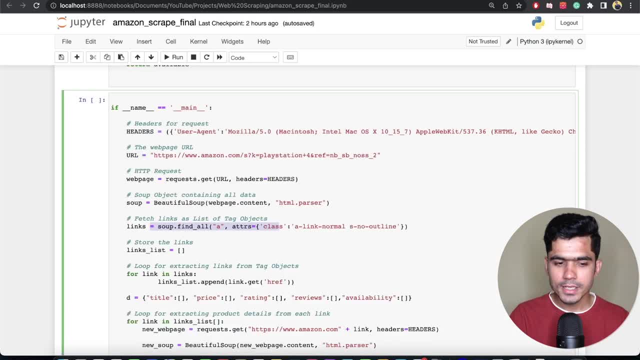 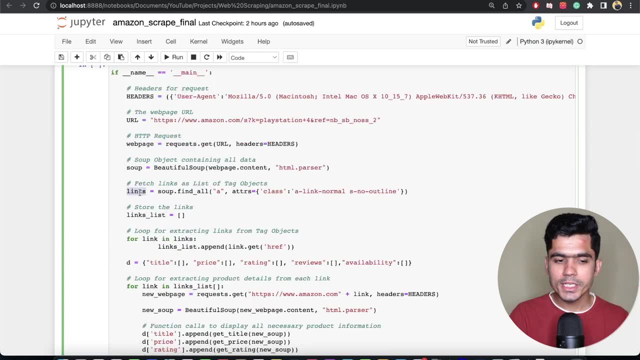 of these links: okay, inside the list, so we are getting it. then we are defining linked list: okay, to store each and individual href tags. so what we are doing is looping through each and every link from this particular list and then appending href. so link dot get href into this linked list. so if you print that, you will only 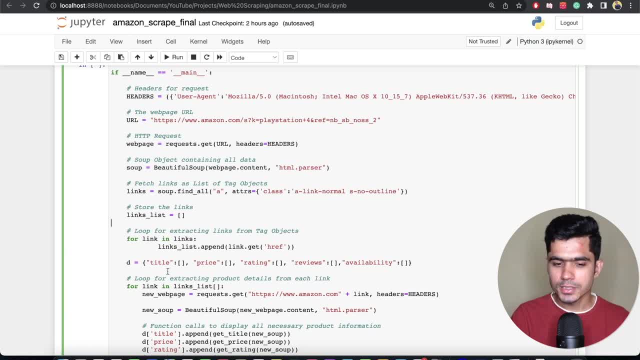 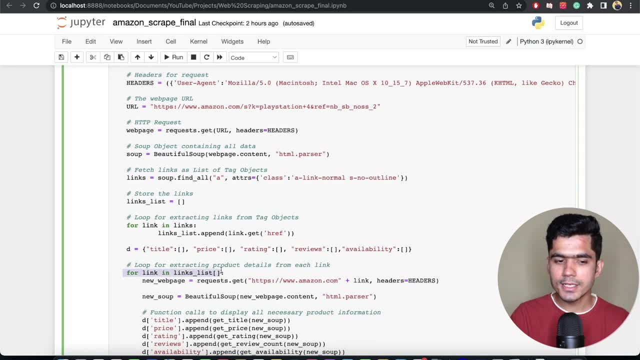 the actual link, then we are defining dictionary. we will come back to this, this part, uh, when we are actually on that. second thing we are doing, doing over here- is going through each and every link, uh, that we just appended, and then we are sending requests to the amazon website again. we 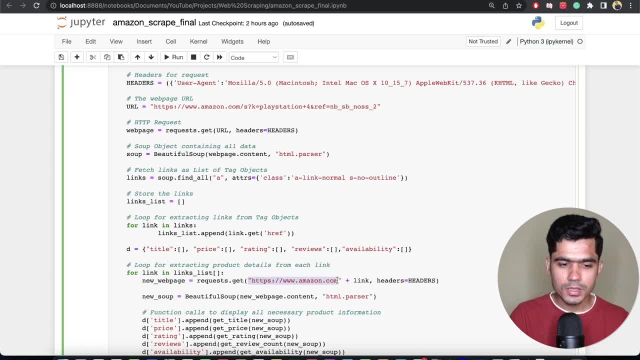 are concatenating amazoncom with the link. so the thing that we did over here, like amazoncom plus link, this is same, but this is inside the loop. so the uh new page, we are assigning this link and we are directly getting the result. and then we are doing the same thing, parsing the html link. so 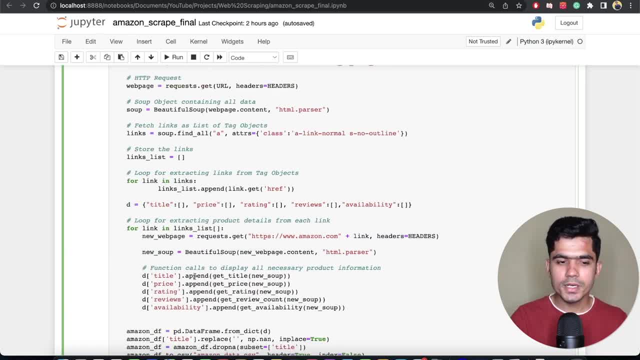 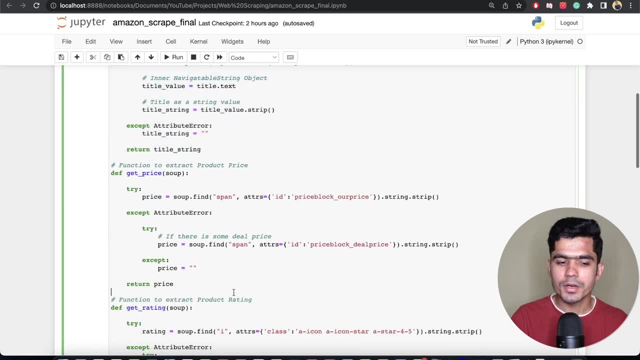 this thing we already did. now, instead of doing everything one by one, what we did is we defined function for each and everything. we did define the function, such as get title, get price, get ratings, get review counts, get availability and all of those things, so you can create your own function. 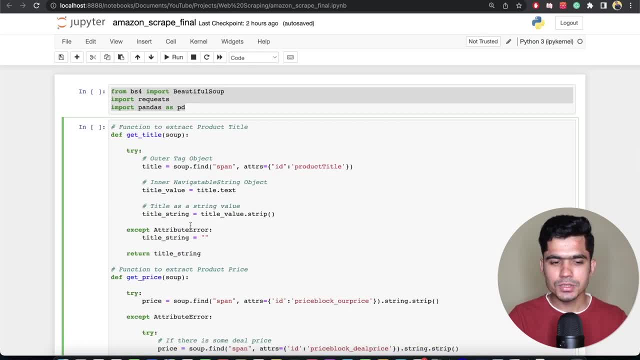 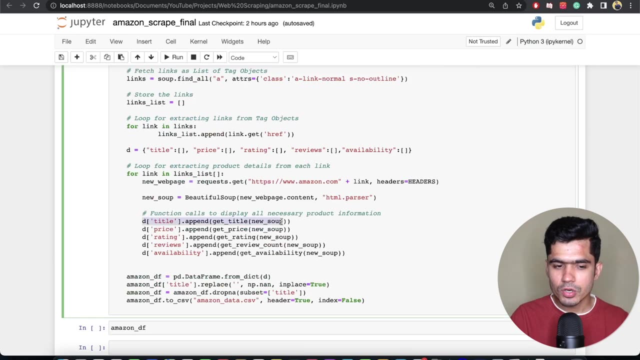 like this. so i will explain you one to two functions and then you can explore the code by yourself. i will put the code link in the description so you can go and check it. but the main important part over over here is that like get title. so what we are doing is we are sending the soup information such as get title, and we are calling. 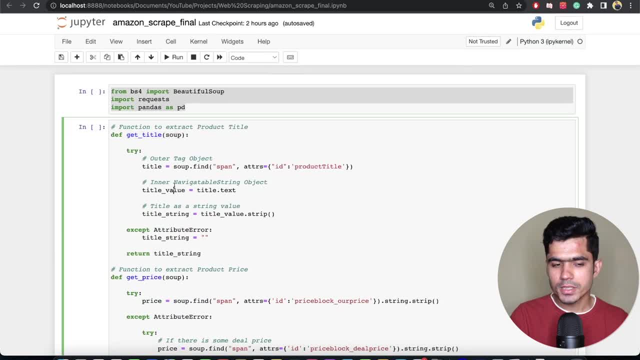 the function. it will call this function. if you understand the basics of python, then you will know that this is the argument. we are writing everything into the try catch. so let's say, if it is not able to find the product title from the amazon website due to some bug, then it will raise. 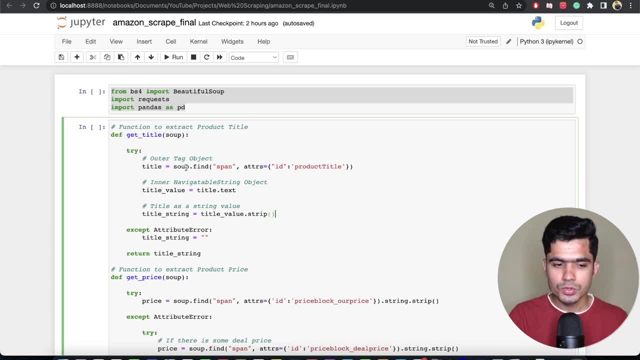 an exception because it is not able to find that product title. so it will go inside the exception and it will keep string as empty and it will return the product title. and it will return the product title, the empty string. but if it, if it is able to find the text information, then it will get the text and 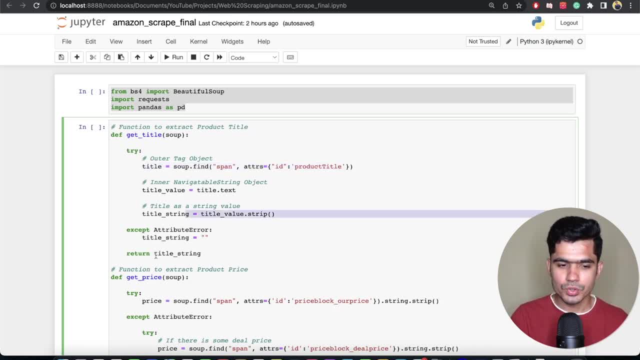 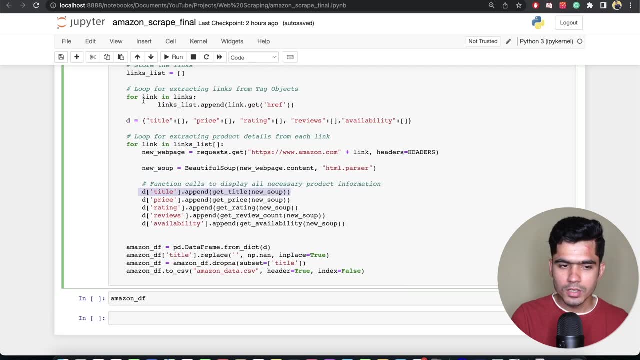 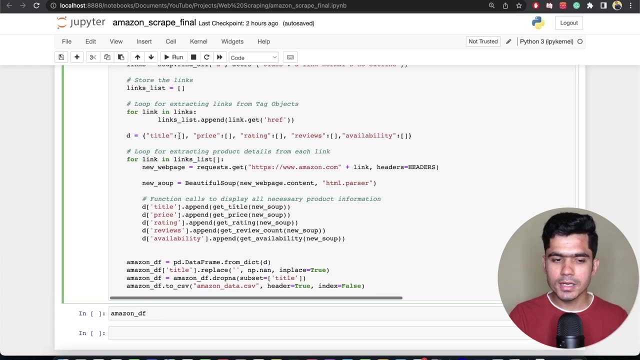 it will strip the value and it will return the title of the string so you will be able to append this title inside the dictionary that we defined. so this is a dictionary d for each and every element that we are extracting- title, price, rating, reviews, availability- for each and every key we are creating. 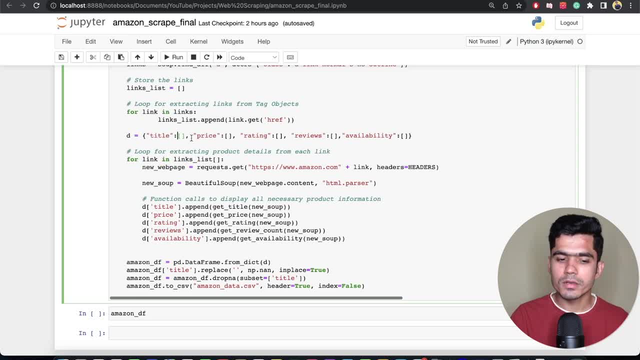 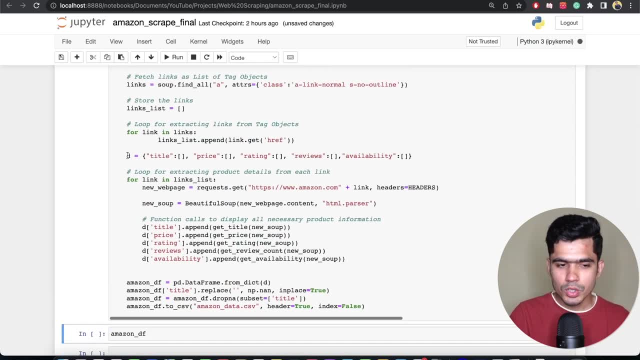 a list and then we are appending all of this element one by one. so let me just run this code until the code runs. let's understand what we are actually doing. so what will happen is that it will go through each and every link and it will append all of those elements inside this list. so title: 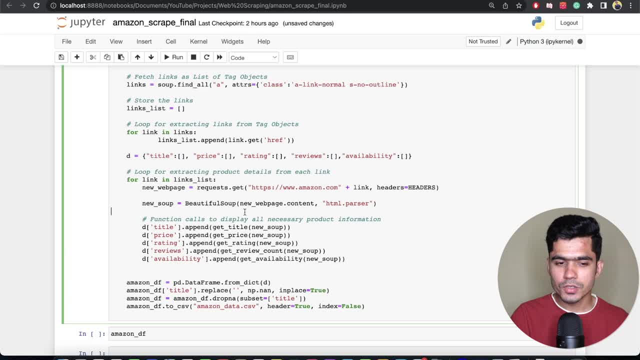 will have one complete list of titles. price will have one complete list of prices. all of those elements will get appended to it. then what we are doing is we are using pandas data frame and using from dict function to build the pandas data frame. so you can directly build pandas data frame from. 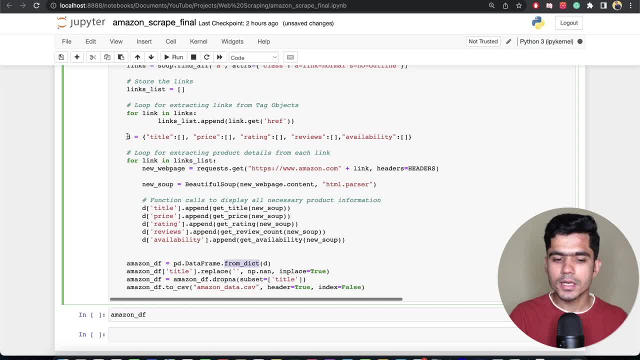 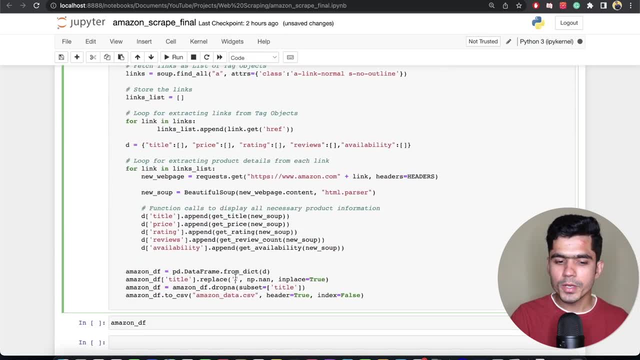 the dictionary or so if you find dictionary format like this, it will directly create and convert it into the pandas data frame. second thing: what we are doing is we are replacing empty value with the null values and then we are dropping all of the null values wherever we don't find the title, because if we don't have the title, 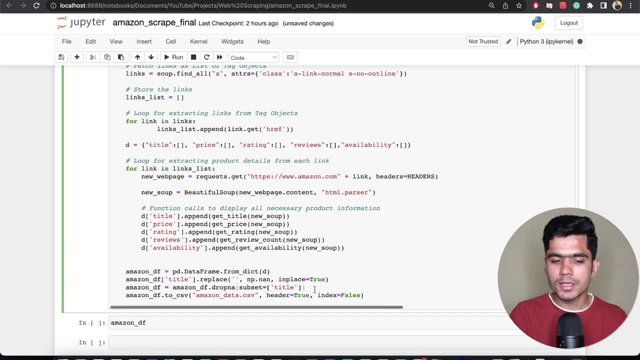 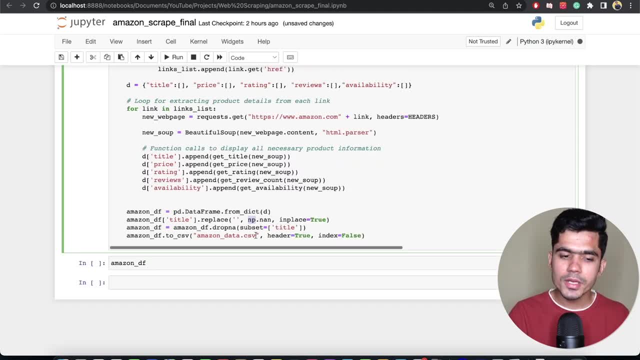 then it doesn't make sense. so we're replacing value with the nulls and we are then dropping those null values and we are storing the amazon data into csv format. one thing you also need to install is numpy library. so while i was running this code, i got the error because i did not. 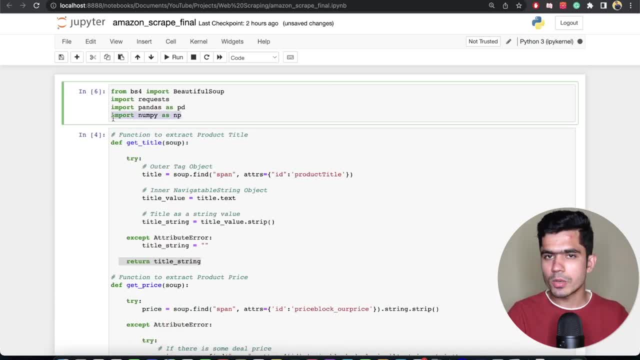 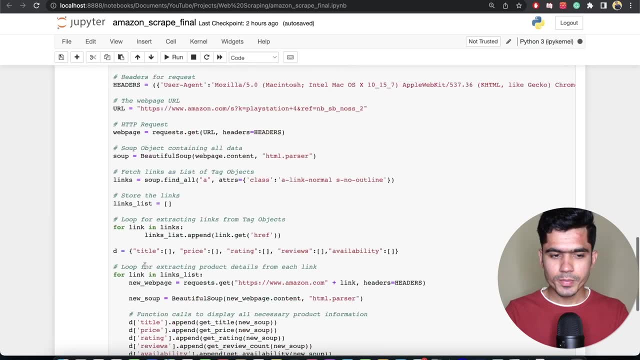 import the numpy. so all you can do if you don't have the numpy, you can just install pip, install numpy and import named as no here and run the code again and let's just wait for. so my code ran successfully. let's just start printing some of the things. let's just print the.